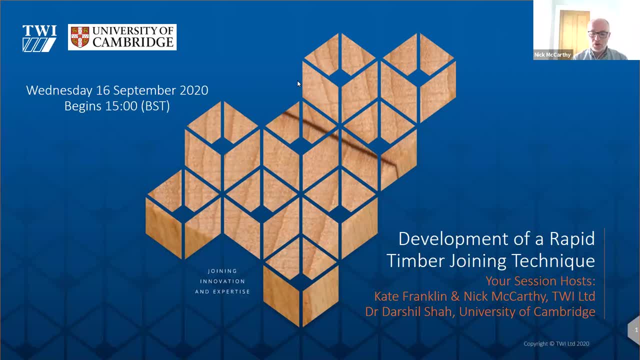 extend a sort of warm welcome to TWI members. I believe there are quite a few that have registered to join the webinar. We're very grateful- and also to the non-members who are joining the webinar today. Obviously, this is the webinar is entitled: the development of a rapid timber joining technique. 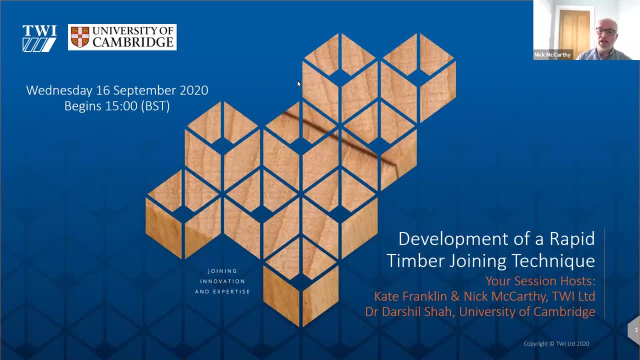 I'm joined by two co-hosts today. We've got Dr Kate Franklin, who is a senior project leader at TWI, and Dr Darshal Shah with us today as well, from the University of Cambridge, And Darshal is a lecturer in the Department of Architecture. I'm sure they will give us more. 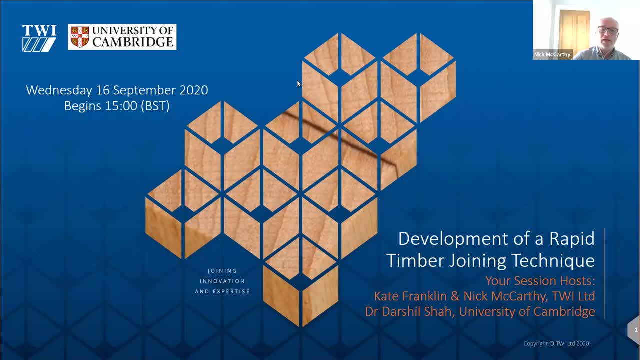 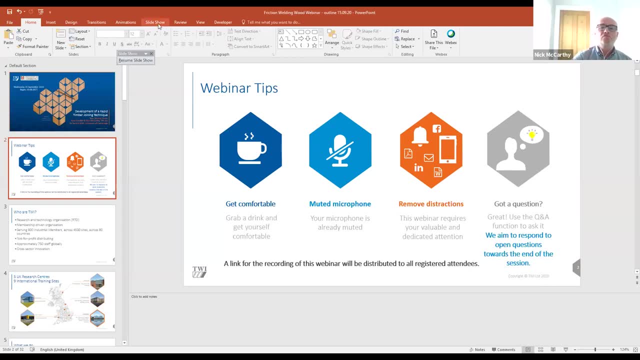 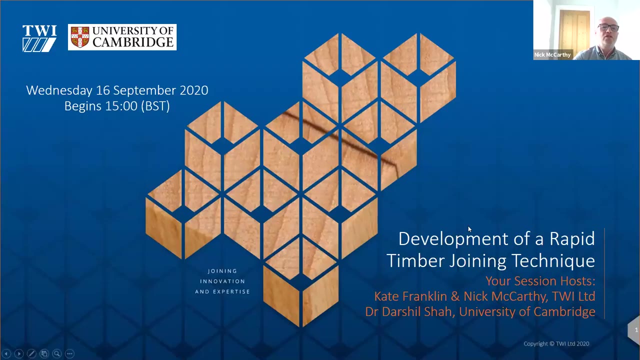 information shortly on where they're at. A couple of points that. Sorry, Kate, can you just start the or can I control it from here? I'm excited to Thank you. A couple of points, a couple of tips that we'd like to. 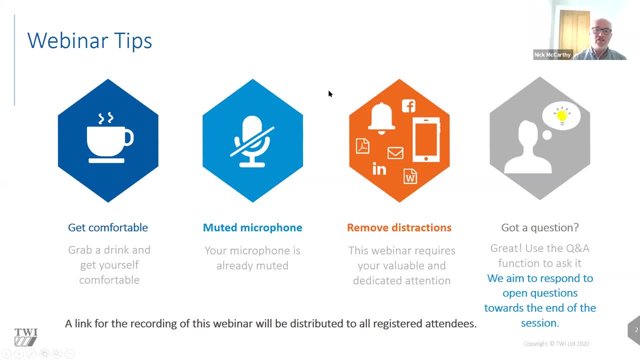 go over before we actually get into the webinar. proper is: get yourself comfortable and get a. get a beverage of your choice. I'm drinking good old, healthy water. Make sure you've got your microphones muted, although they should be by default, I think, when you join the webinar. 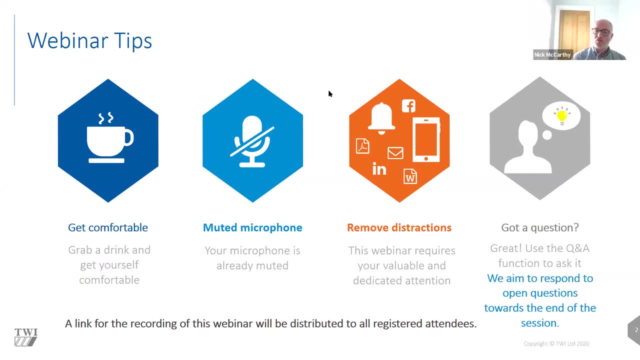 Remove any distractions such as, you know, iPods, phones, etc. etc. That'll be good, unless, of course, you're watching the webinar on it, which wouldn't be good. And if you've got any questions, great, we welcome those questions. We'd ask you to use the Q&A function, which you should be able to access. 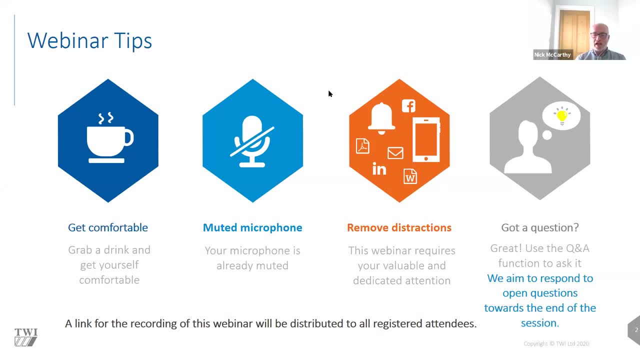 I believe. I think it's at the bottom of the screen. Obviously, we'll aim to sort of answer those questions at the end of the webinar. Rest assured, if you ask a question and we don't have the time to answer it at the end of the webinar, we obviously are recording the questions. 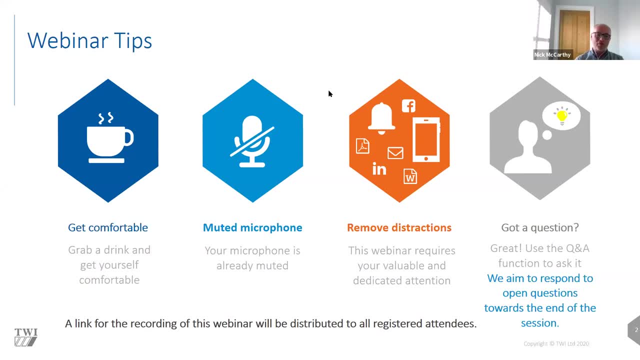 As well, and we will get back to you in due course, after the webinar. We'll be back in contact with you And, as I said at the beginning, you know there will also be a link of the recording of this webinar which will be distributed to all the registered attendees as well. 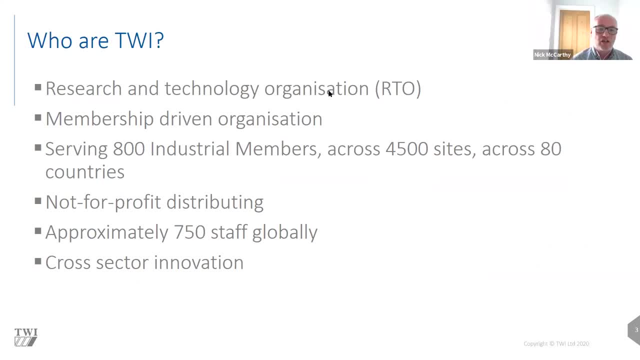 So what I'd like to do first of all is for those who aren't familiar with TWI- and I do appreciate, perhaps you know, because of the application we're talking about at the moment, quite a few people might not be familiar with TWI. I'd like to give you a little bit of an overview of who we are and 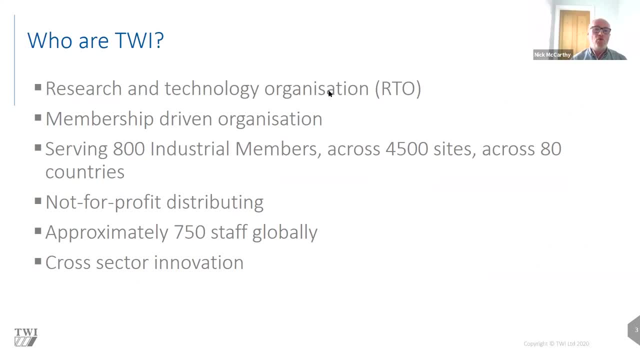 what we are and also, of course, where we are and what we do. So we are as the slide says. we're a research and technology organization, an RTO. We are a membership driven organization. You're basically working with the TWI. Membership is a requirement. We're a membership driven organization. 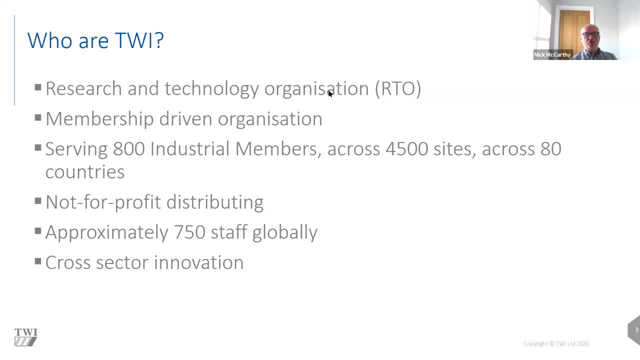 You're basically working with the TWI. Membership is a requirement, Obviously. that membership has numerous benefits, of which we'd be more than happy to go into on perhaps a different meeting at a later stage if that is of interest to you. But you know, as a rule we're actually currently serving. 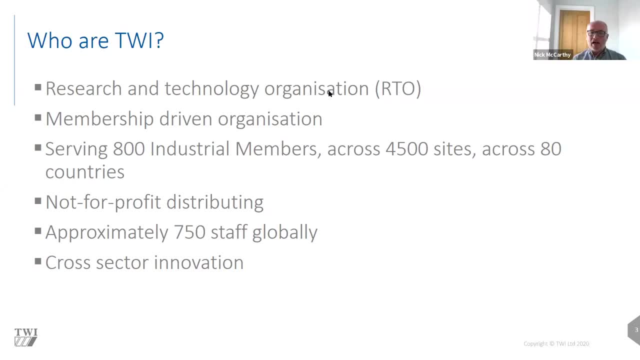 around about 800 industrial members And, as you can see from the slide, those are spread all over the world. Obviously, you know we have quite a large membership in the UK But, as it says, you know, there are approximately four and a half thousand sites across 80 countries. 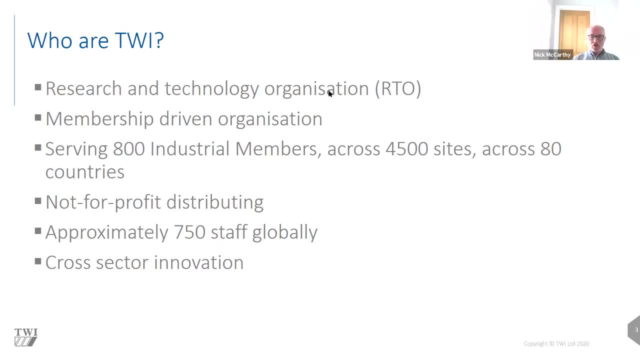 worldwide. We count a lot of very big global companies within our membership and we would be. we'd be talking companies like Boeing, BMW, sort of Shell, Rolls-Royce, But right the way down to SMEs and smaller companies. So we work with a broad spectrum of companies and we also work. 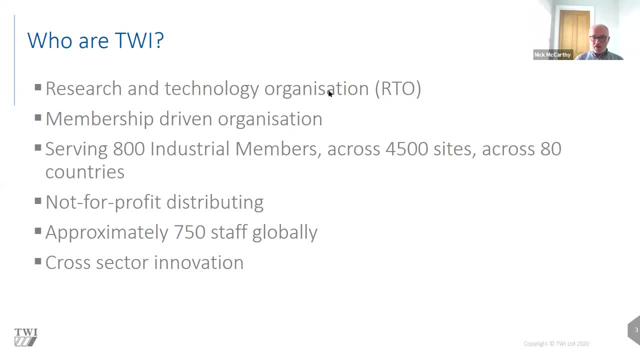 across a broad spectrum of companies. So we work with a broad spectrum of companies and we also work across a broad spectrum of companies and we also work with a broad spectrum of companies and we also with a broad spectrum of companies and we also work with a broad spectrum of companies. 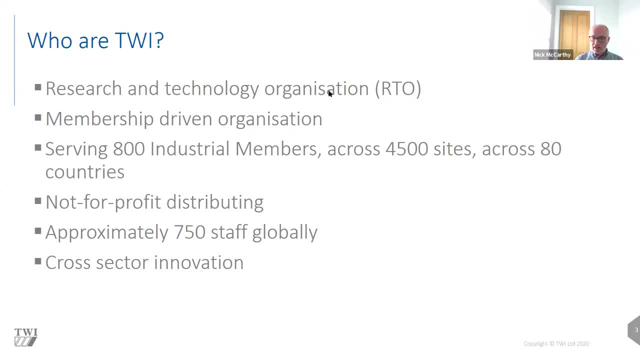 We've tended to work a lot in the oil and gas sector historically But you know, in recent years that has diversified and we're working a lot in other areas as well. We are, as it says, not-for-profit, distributing. Essentially, as I said, it's very much an organization which is driven by its membership. 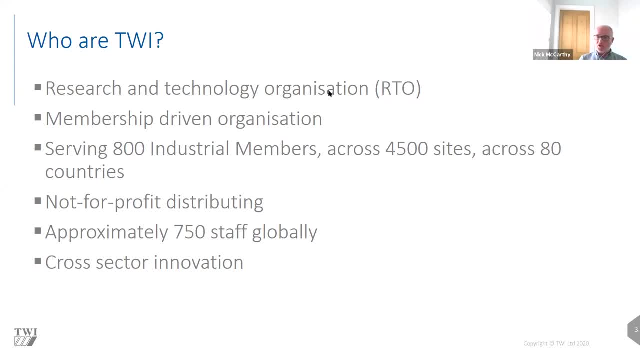 When you join TWI, a percentage of your membership goes back into what we call the CRP or the course research. So that's the more of a general approach you know. you know, for example, our benefits in the industry, So that you have a really broad spectrum of companies and we're not just 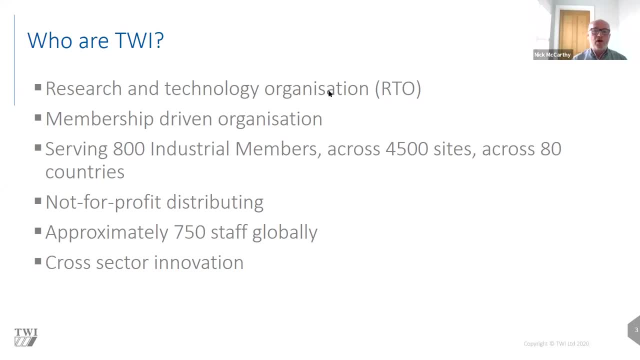 program um. we have approximately 750 staff globally um. quite a few of those are based in the uk, but but then, as i've also said, we have offices um dotted around the globe and in those offices are obviously staff supporting training and other activities as well. and it's important to say that, to underline that cross-sector innovation, because of the, the range, 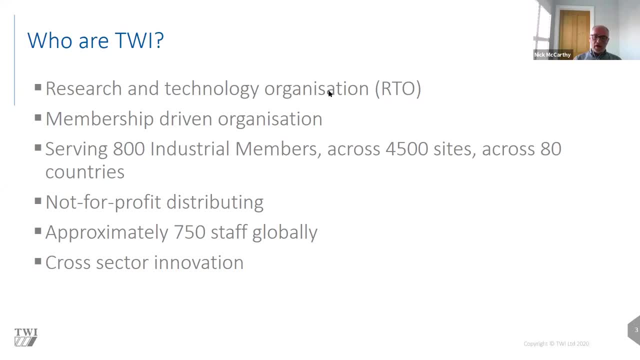 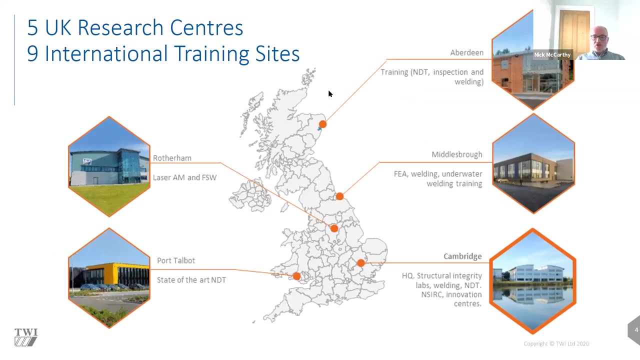 of technologies that we deal with at twi. um, you know it obviously appeals to a lot of different sectors. um and um you know, we'll perhaps touch on some of those in a bit. um, so, as we've said, we are, um we're focused out of the uk, the headquarters there, which, in fact, is where i'm based. 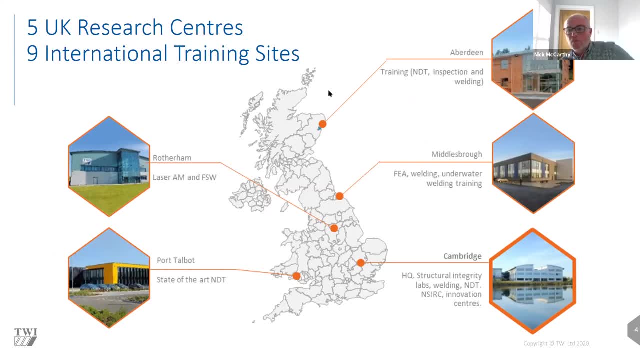 and it's also where kate currently is. i'm um, as is probably, with a lot of people. we are some of us who are in the area we're in, but we are heavy in our facilities so we're not going to be a lot of people at the moment there. so it's part of the the the current situation, um, but it's important to. 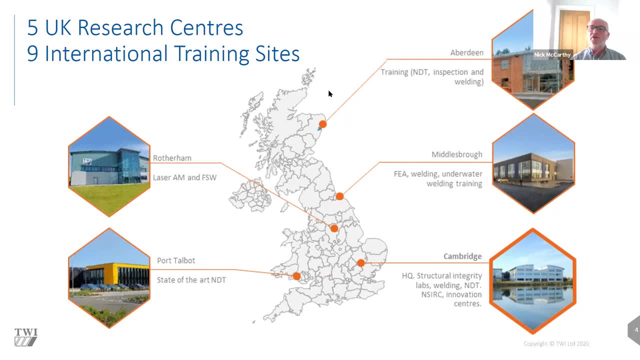 underline that, for instance, on our facility in cambridge, where it's obviously safe and proper to do so, we are continuing to work um as much as we can, as normal. so the labs are all still working, et cetera, and i think darshal is probably in cambridge as well at the moment. so, um, that's where. 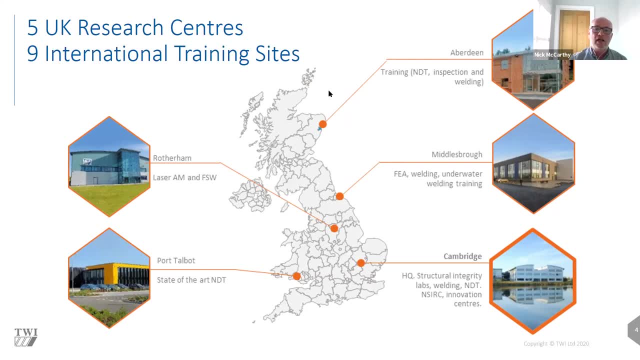 there. but you can see we are spread across the UK. For instance, if we look at the Aberdeen site, I already mentioned that we do a lot of work with oil and gas, for instance, and obviously from the UK that is a key centre for oil and gas. So we have a training centre and NDD. 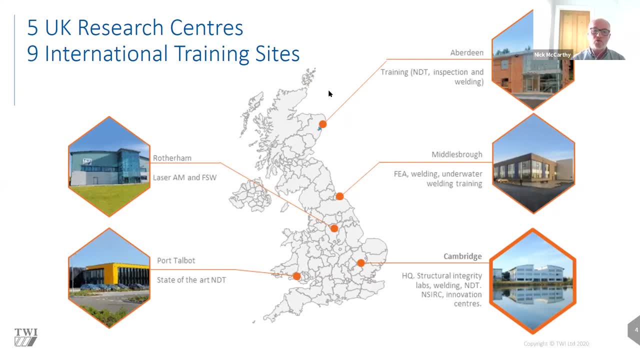 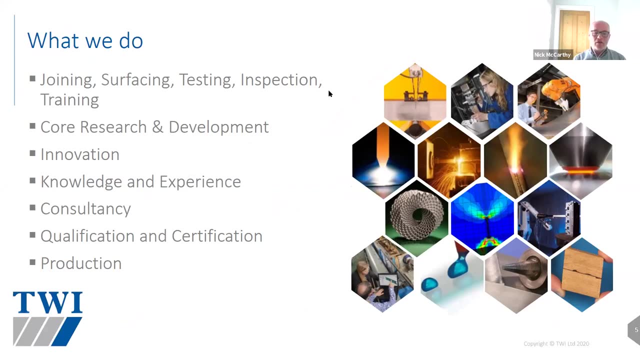 inspection and welding expertise there as well. So what do we do? Well, TWI, the welding Institute, was set up in 1946. Because of the name, people automatically think of us for welding and joining, and that's absolutely fair enough. We certainly want that. we don't want. 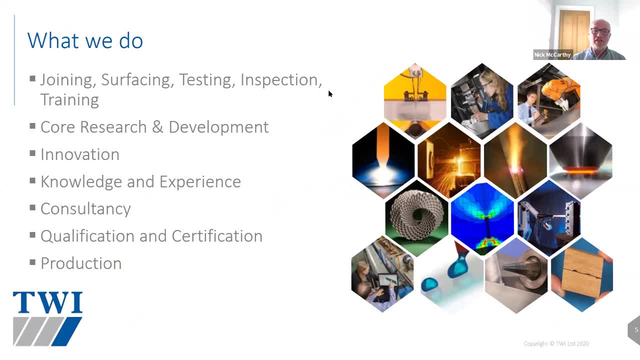 to change people's opinion there, but we actually do so much more. We have diversified into so many different areas and so many different technologies over the years. um so, yes, we do joining, yes, we do surfacing, we do testing, inspection, training and a lot of other things. 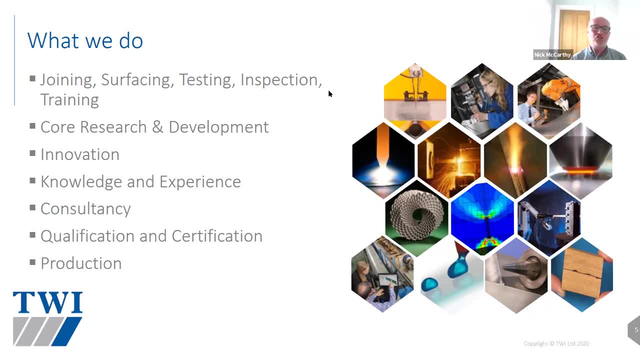 even welding wood, which we'll talk to you about in a short while. um, i touched upon the core research program that we have. we're very, very focused on innovation and development, so we'll show you a little timeline shortly of what twi has has been involved with since its inception. um, i guess one. 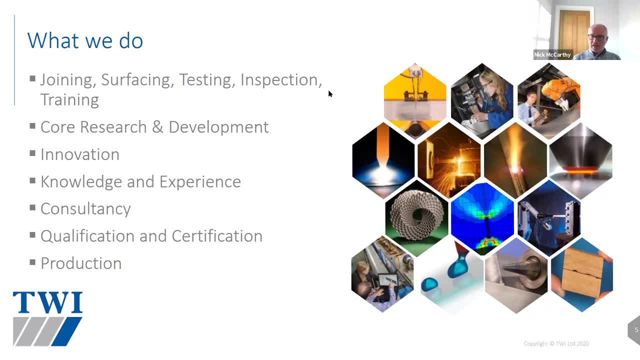 thing that i would like to highlight would be friction stir welding, which is a technology that was was developed, was invented by twi and has been developed since then. um, and that's been a very, very important technology for use, for instance, in the in the electrification ev market. um, it's used. 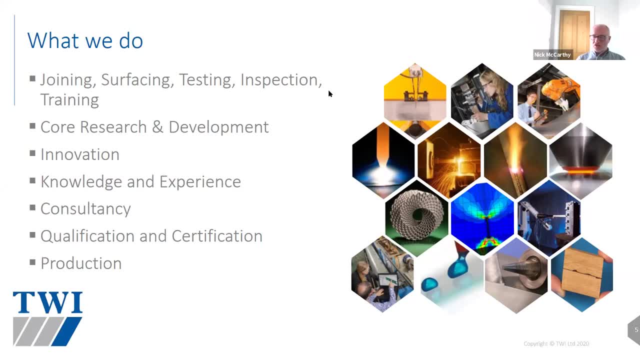 um battery technology, etc. so and obviously used in aerospace and a wide variety of different applications. so i'm very proud of the fact that we've- we've, you know, we've- invented technologies like that and the fact that we continue to innovate with technologies. um, so twi has a wealth. 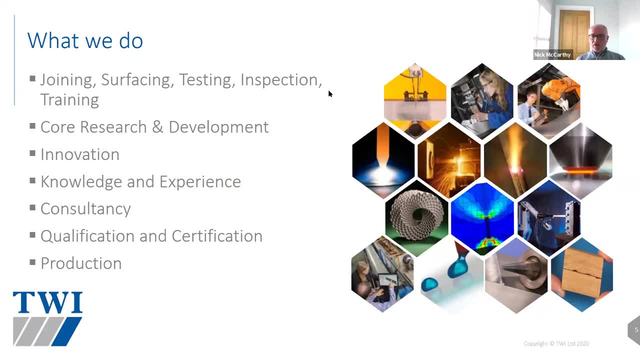 of knowledge and experience. um, a lot of very clever people, a lot of people very, very focused in their, their field of expertise and they're very, very focused on the technology that they're using and they're very, very focused on the technology that they're using. um, so twi has a lot of. 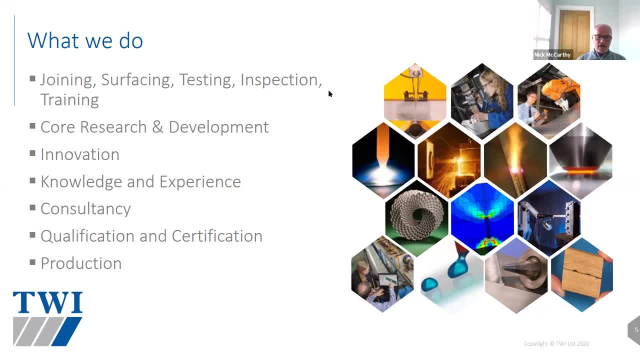 knowledge and experience, um, and as a result of that, we we work with companies where we're we're looking at products from from sort of inception right the way through to production, um, and we work. it's important to underline, for instance, we also work closely. we have in membership, a lot of 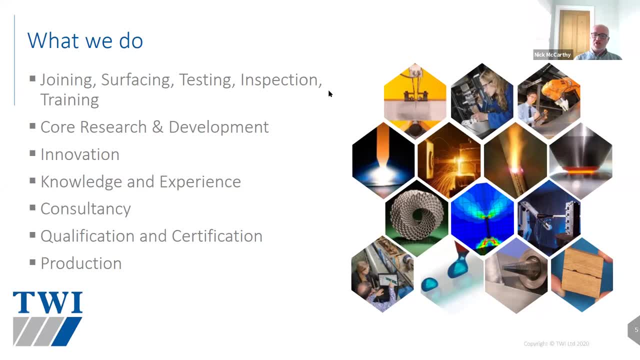 the supplies of the equipment that companies will use to go on and manufacture the products that we're helping them develop. um, obviously we've got a lot of technology that we're using to, and obviously we we also uh count qualification, certification, training that i've touched upon. 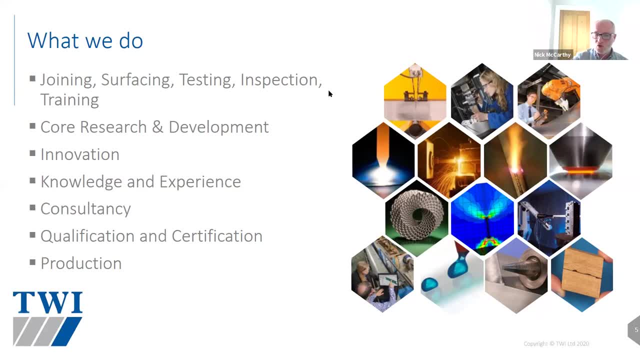 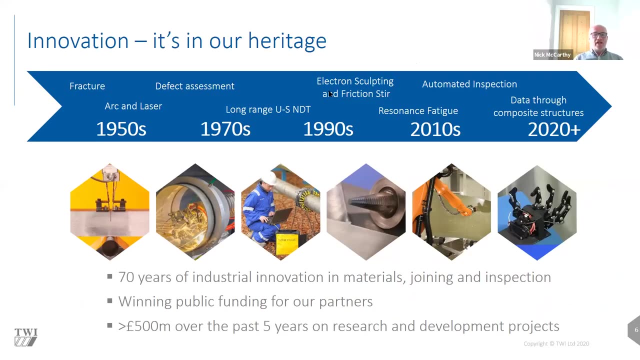 and even um on occasion, we will get involved in production as well, um where it's right and proper to do so and and where we can't offer that service via one of our members. so, um, that's a little bit of a timeline there, really covering um the 70 years or so of the, the innovation, um. 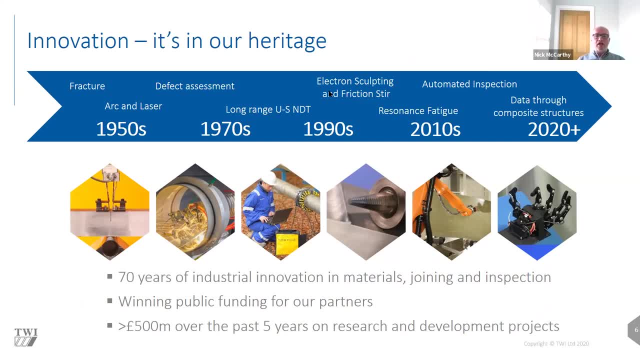 materials joining an inspection that we've had at TWI. You know a few points that we'd highlight. there is the- as I've already said, it's friction, stir welding, electron sculpting- Right the way up to 2020, we've been working with things like data transmission through composite structures. 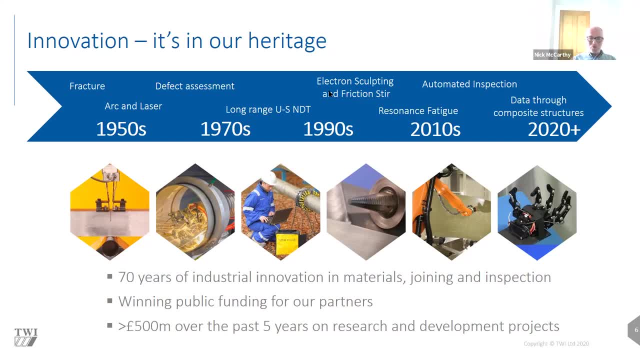 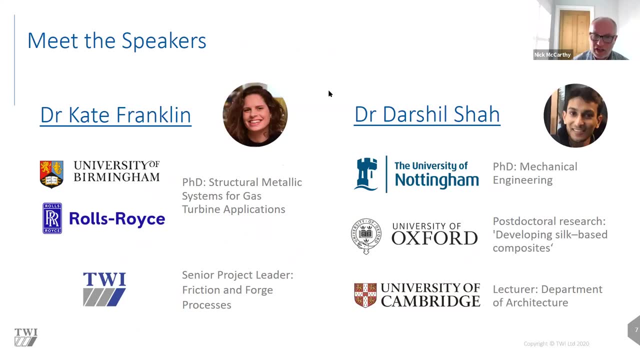 which is a really, really exciting prospect as well. Thanks, Kate. Okay, So the two speakers that we've got today very, very pleased to introduce you to Dr Kate Franklin. As I said, Kate is a senior project leader in our friction and forge processes section. I mean just to give 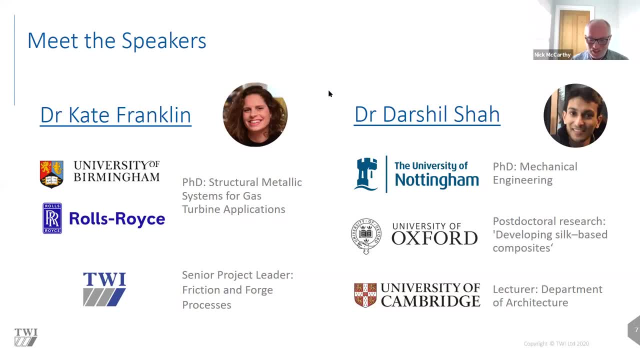 you. my name, by the way- sorry, I should have said this at the beginning- is Nick McCarthy, and I'm a business development manager for the advanced manufacturing technologies group at TWI, And within that group we have several sections. One of those sections is friction and forge. 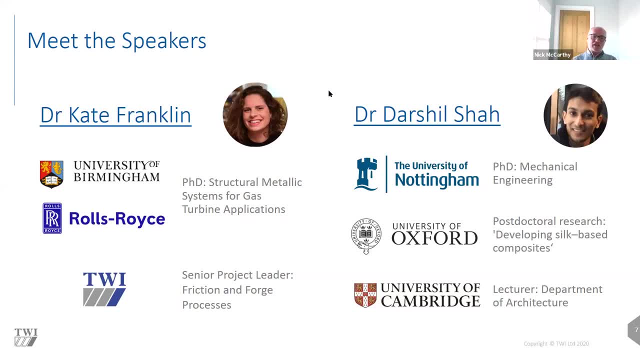 processes And Kate works within that section. Kate studied at the University of Birmingham and also has a PhD in structural metallic systems for gas turbine applications, which was sponsored by Rolls-Royce, And obviously, as you can see, Darshil, who I'm sure will. 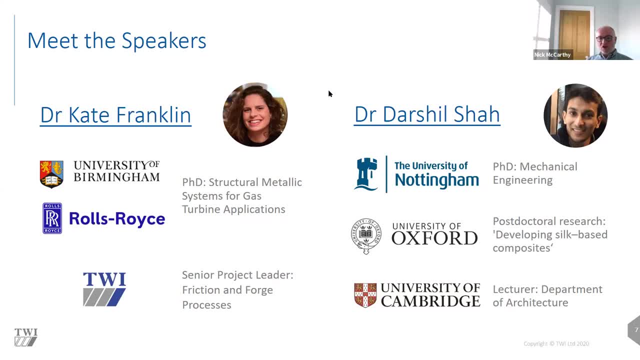 introduce himself as well, but is a lecturer in the Department of Architecture at Cambridge And I know has a number of other strings to his bow as well, which I'm sure he'll tell us about shortly. So I think I'm going to hand over to Kate now, who is perhaps going to give us a bit of. 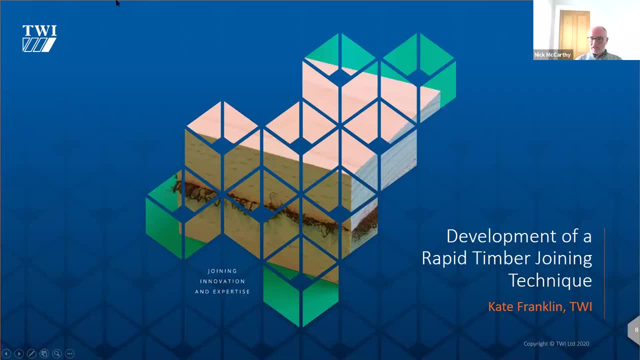 background in the technology that we're using, the process that we're using, the established technology that we're using for this process. So over to you, Kate, Thank you. Thanks, Nick. So yeah, as Nick said, I'm Kate Franklin. 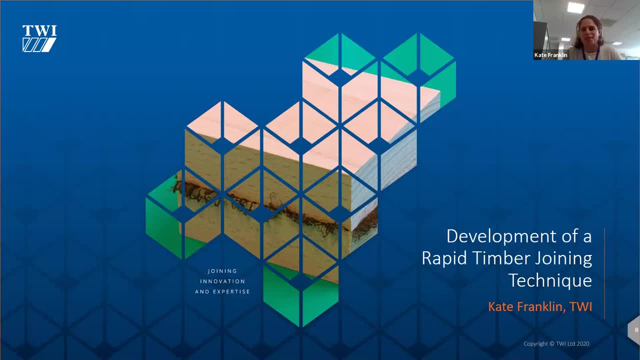 I'm working here at TWI. In fact, this is the first day I've been in the office for six months now, So it's a very exciting time day for me. So when I normally tell people that I work in welding, they often think that I wear like a mask and have a little torch, like in flashdance. 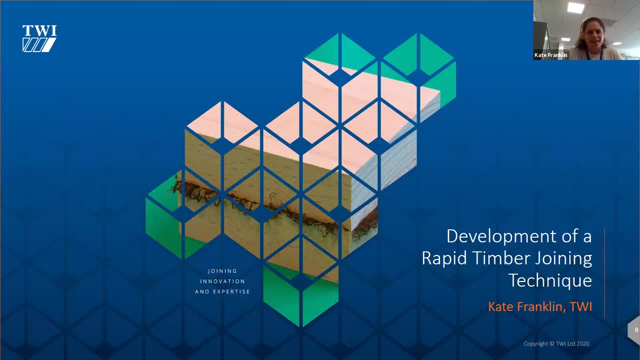 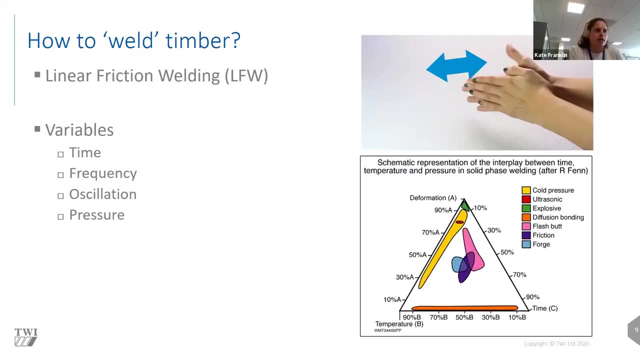 and I have to disappoint them pretty quickly, And so my PhD and my work here at TWI is focused on friction welding. So just a little bit of what is friction welding and how are we using that to join timber? Okay, so in this instance we're utilising 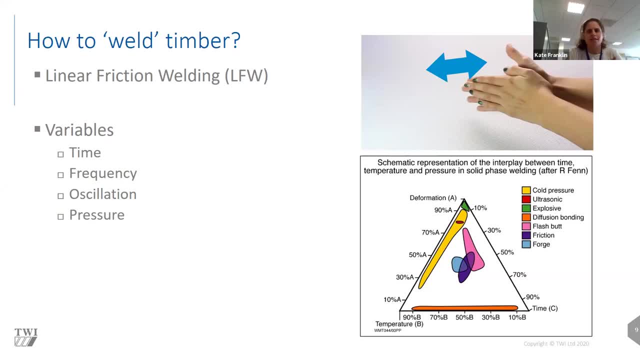 linear friction welding, which is essentially rubbing two parts together. So I'm holding one static and rubbing it. So there's in metal. there's no melting involved. the temperatures remain really low, which means that it's a highly controlled process. 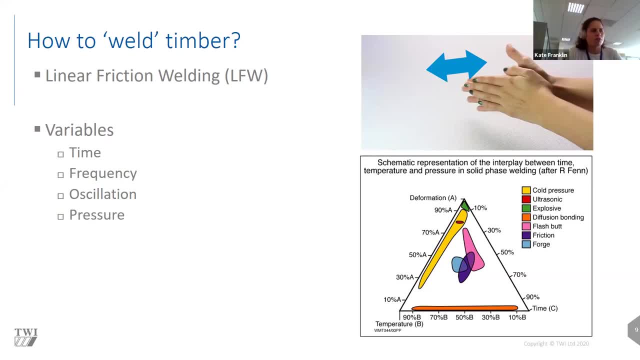 a mechanical process that's got really high repeatability, no melting, And there's a few variables with that. So we can, obviously we can- change how long we run that process for the frequency and the oscillation of the movement and the pressure. 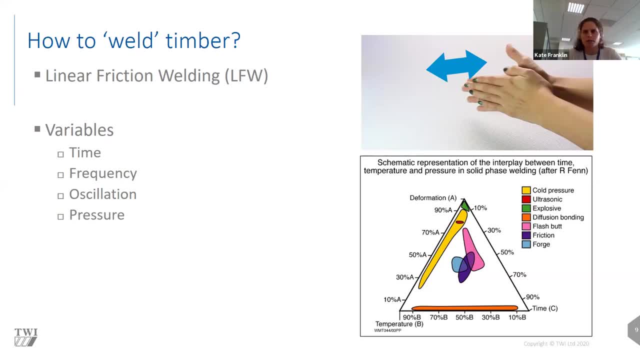 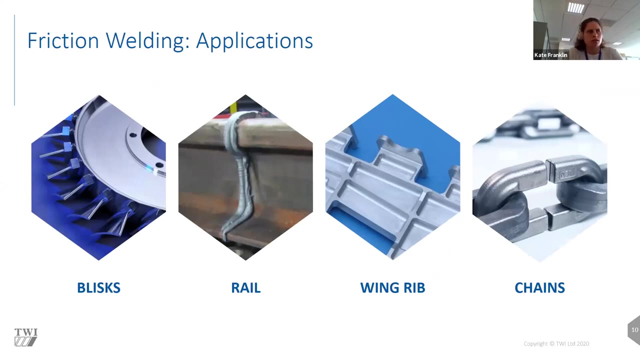 So how hard we push those two parts together, And I'll explain a bit more about the process in a later slide, But I just want to highlight the applications where this is used and what the advantages are. Okay, so friction welling is normally used in safety critical. 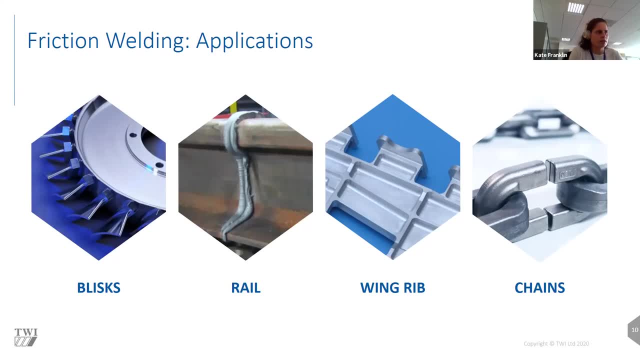 applications where high quality is really imperative. So, like I did my PhD with Rolls-Royce, that was on friction welding in aerospace engines And an example of that here is Blisks. So you linear friction weld the blades to the larger disc. You can also. it's also been used in rail. 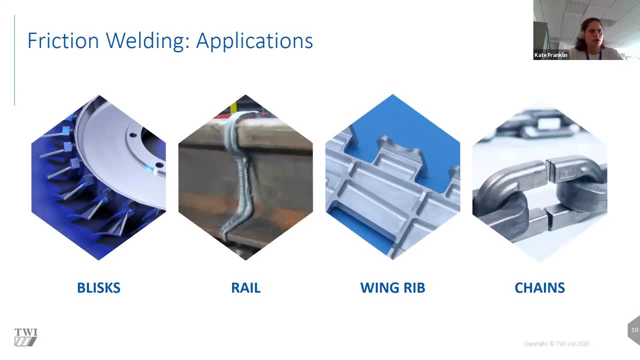 and chain applications, And here I've used an example of a wing rib to demonstrate its use to produce near net shape components Where you're adding something to a thinner part to allow you to reduce the machining on that part. So it's an established, mature technology. 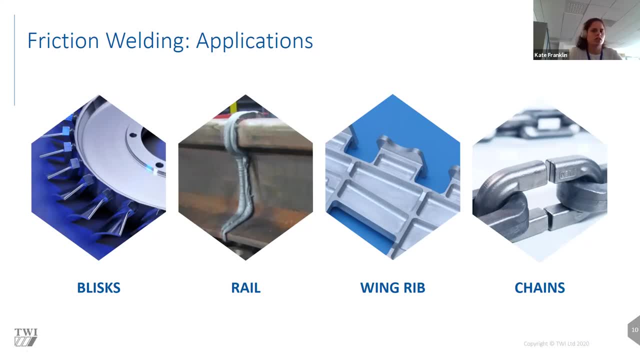 Issues traditionally in traditionally conservative industrial areas So such as aerospace, in planes, rail, And it's tends to be used for safety critical components that require the highest engineering demands. So essentially it's the best type of joint, or at least I like to think so. 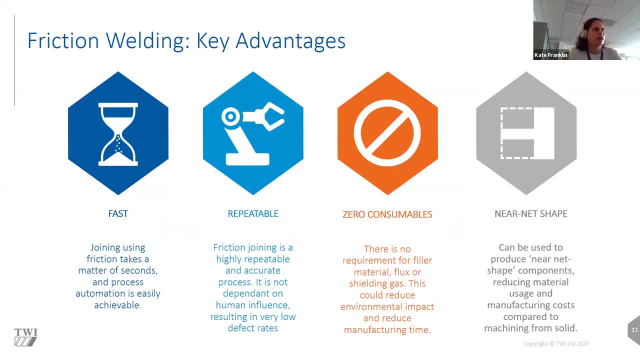 So what are its key advantages? And here I've tried to pick out advantages that I think are key in metallic applications that we normally work in but also translate very well into wood. But also translate very well into wood. But also translate very well into wood. 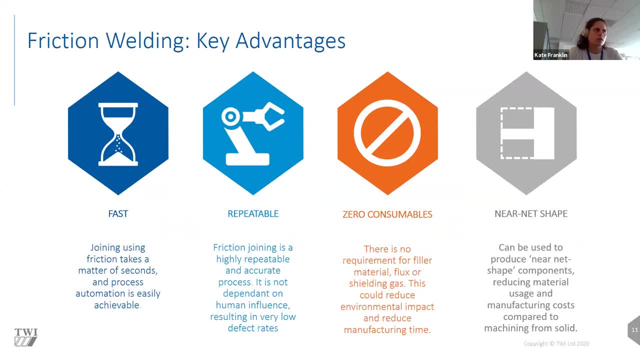 And what we think will be important- using this in the timber industry. So it's incredibly fast, So it takes just a matter of seconds to join the parts. Initial trials that we've done on wood have all taken less than 10 seconds, And I shall talk a bit more about the best times. 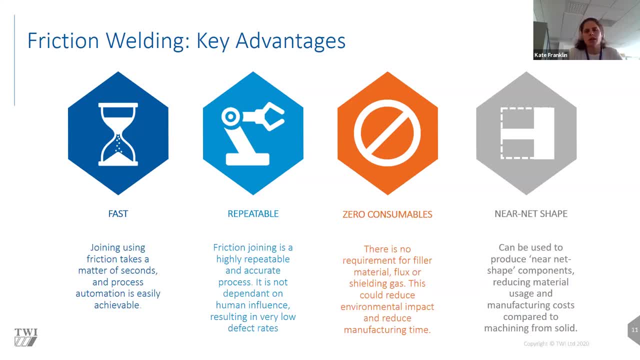 but they're very, very quick And even the entire process as a whole, including moving parts in and out, can be fully automated And therefore just take just a matter of seconds. So in terms of wood, this also means that there's no cure in time. 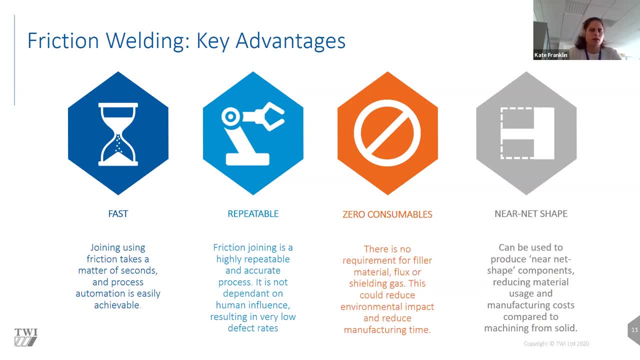 And we're reducing labor costs and time by automating the process. It's highly repeatable, So it's known for its repeatability. Every joint produced is almost identical And, due to the removal of any human influence, it results in very low defect rates. 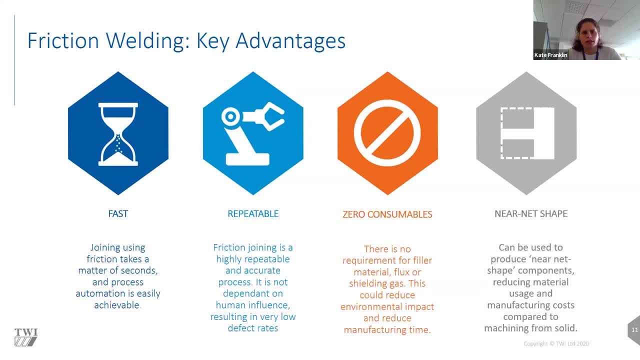 So, thirdly, the process doesn't require any additional material. So in metal that means that we don't use a filler wire or flux and we don't need a shielding glass, And in timber that means that we don't need any additional material. 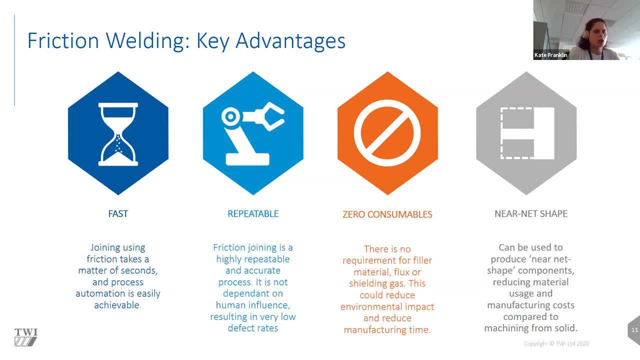 And in timber that means that we don't need any additional material. And in timber that means that we don't need any additional material, Any additives. So no glue, No solvents And there's no need for any mechanical fasteners. 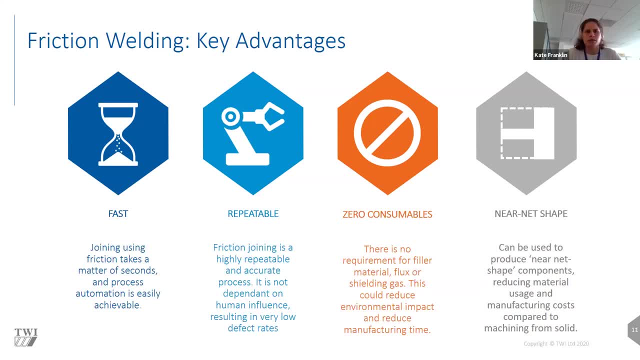 You're removing any additional metal or plastic or any other component that you might use in the joint. It is just timber to timber And we think that this could reduce the environmental impact of products as well as reducing the production time and cost. And finally, it can be used to produce near net shape components. 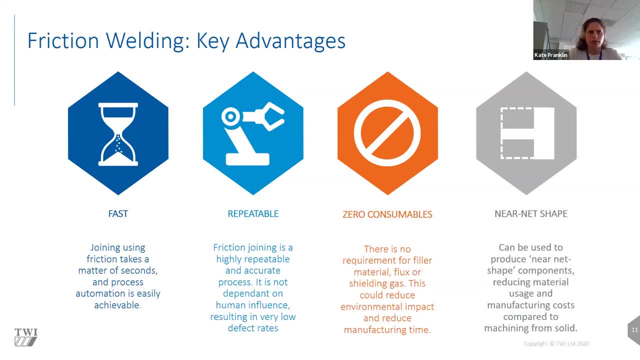 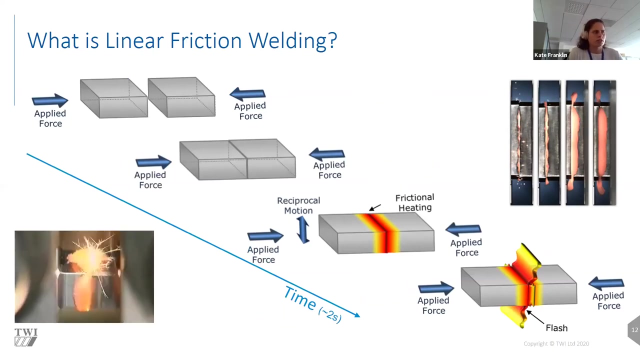 So, as I mentioned previously, this can allow you to reduce manufacturing costs compared to machining from solid. It reduces material wastage and reduces the cost of materials as a whole. Okay, so what is linear friction welding? So I mentioned previously that it's essentially just rubbing two parts together and that there's no melting involved. 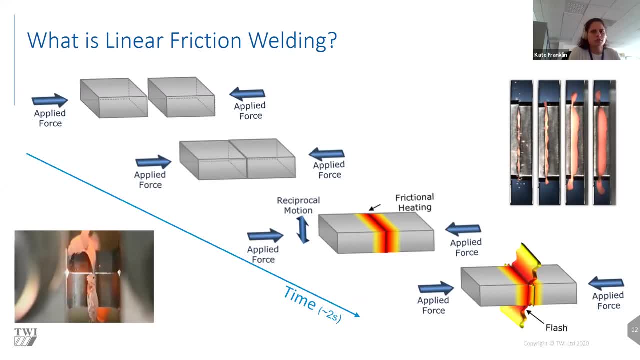 So it's generally termed a solid state joining process. And that's because in metallic materials, the friction is used to heat the interface and allow plastic deformation. and mechanical mixing, Okay, But not melting. And in linear friction welding that heating is achieved through the application of pressure and a linear oscillating motion. 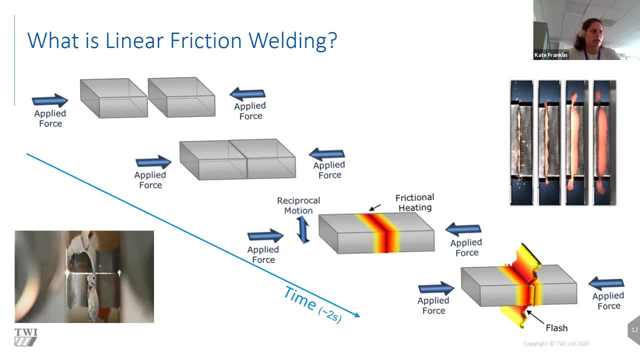 So, as you can see in the schematic on the screen and in the video, one part is held still and they're brought together under an axial force. One of the parts is then linearly oscillated while the other remains stationary And finally the oscillation ceases and a forging occurs. 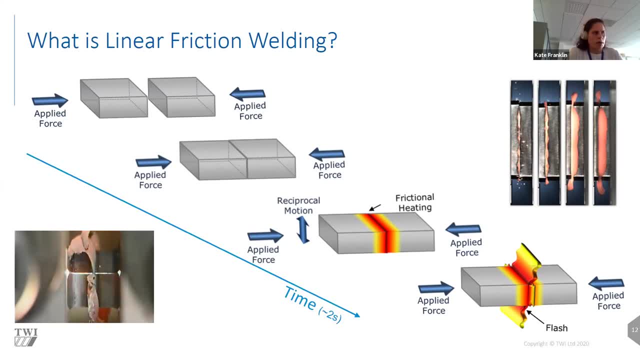 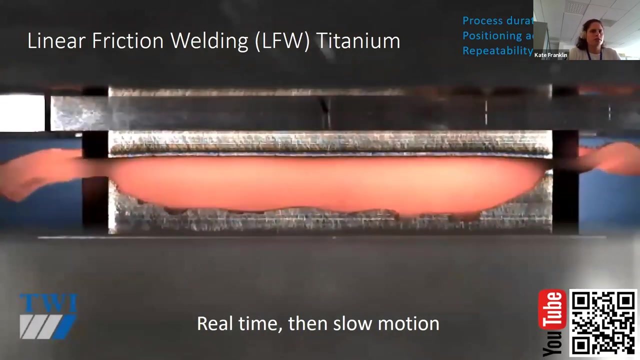 And then the axial force is applied, So they're pushed together. essentially, they're held together under a force once that motion's stopped, And the process is completed in a matter of seconds. Okay, so here is a video of linear friction welding using titanium. 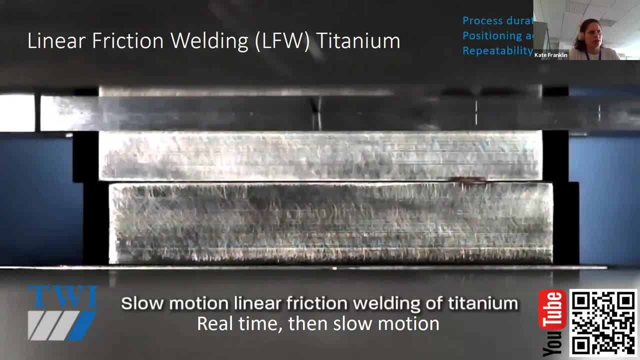 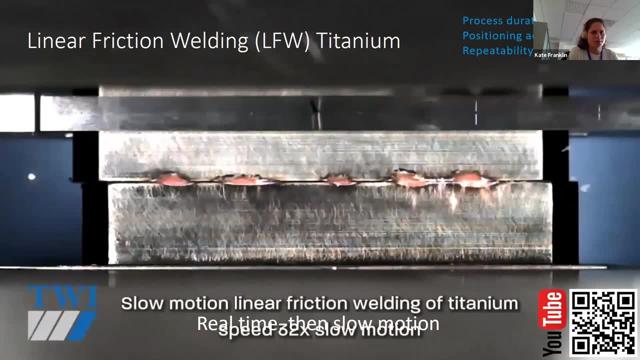 And it produces a joint in just four seconds And you get full consolidation. Now I can see a perfect video in front of me that looks incredible, But I'm aware that, due to bandwidth constraints, you might not be able to see the same quality video that I'm seeing. 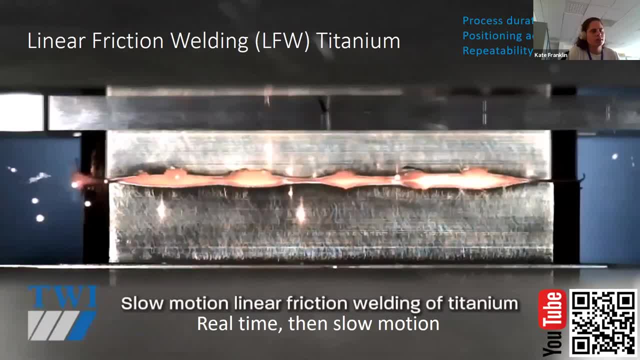 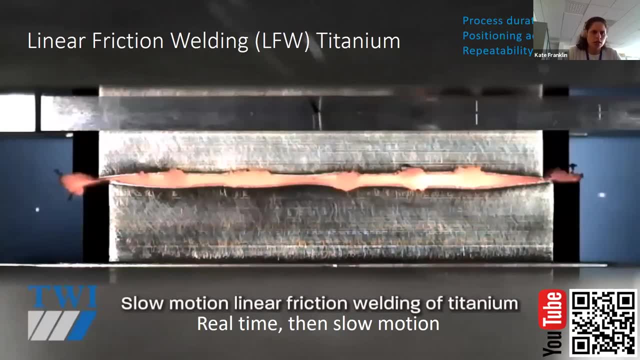 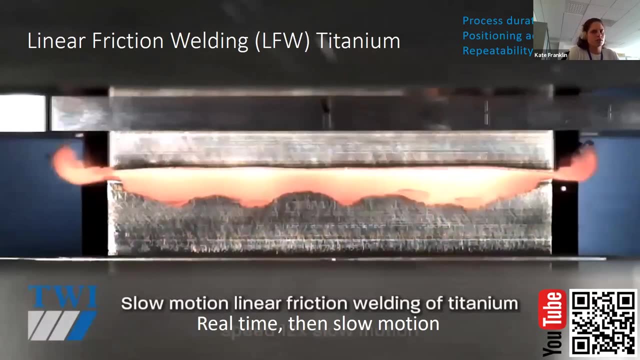 So these videos are available to view on YouTube And we'll send the links out to those. and there's some information on the last slide. Okay, so over time at TDI we've welded A wide range of materials together using this technique. 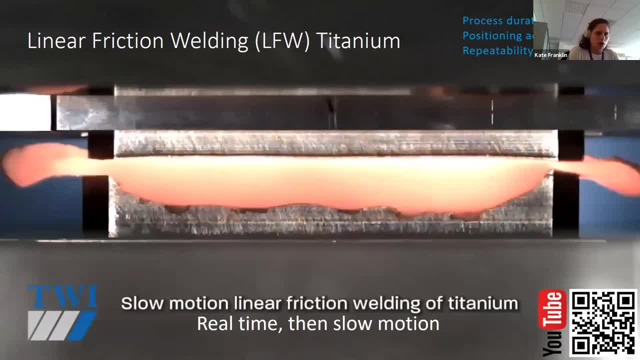 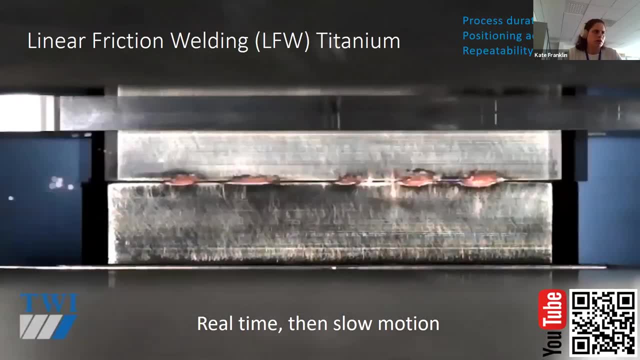 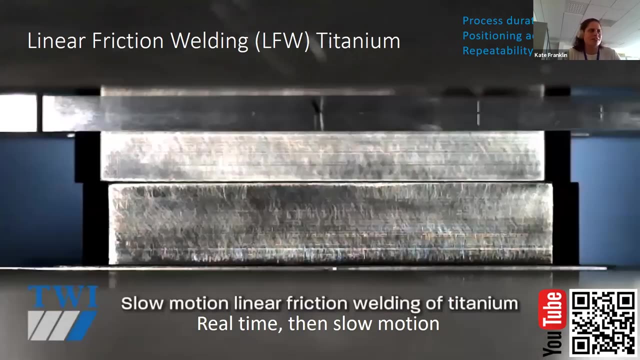 So we've looked at metals, refractory metals, polymers, ceramics, composites, And we've also used the same machine to do testing on rocks, and we've even joined chocolate together, And all of these have had successful results. So we had to work out where to go next. 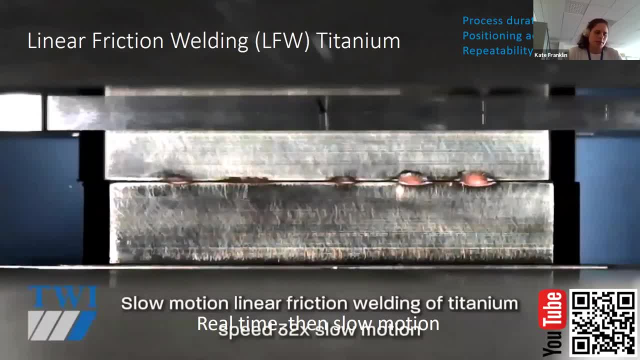 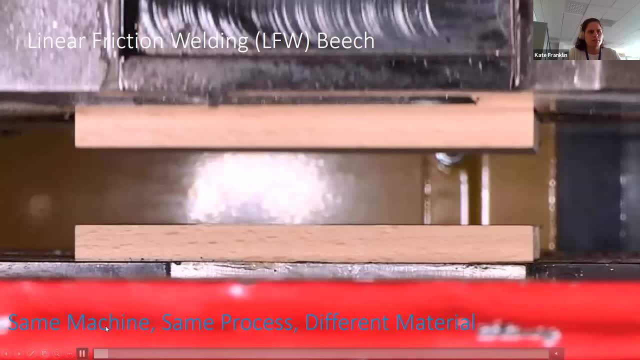 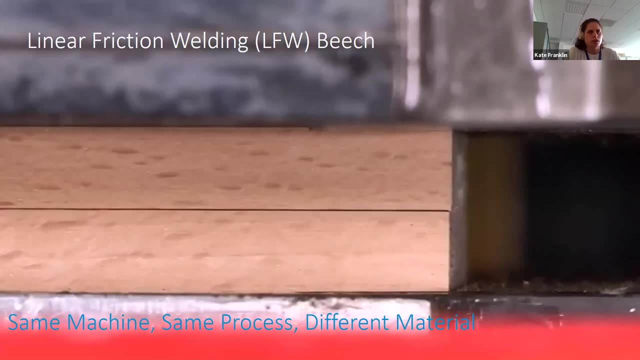 And the latest thing we've tried Is timber Again. this is the same machine and exactly the same process, but now we're using it to join beach Again. the video might not be as good quality on your screen as it is on mine. 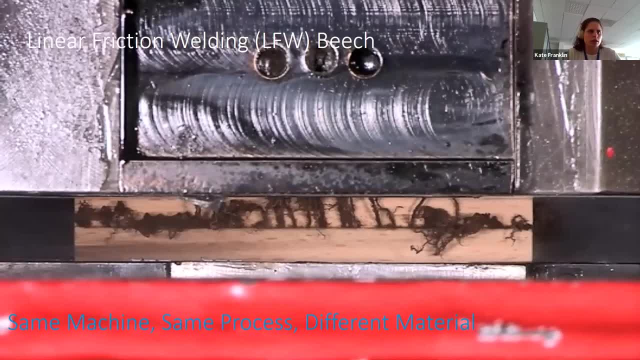 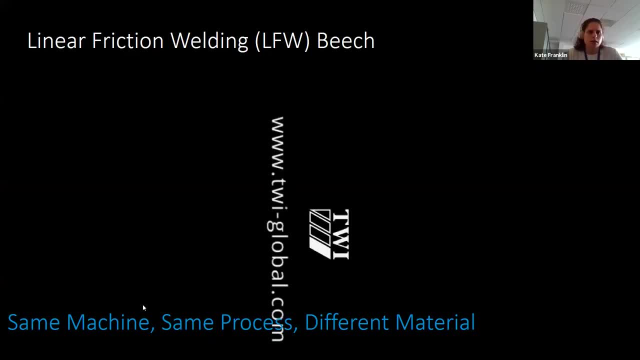 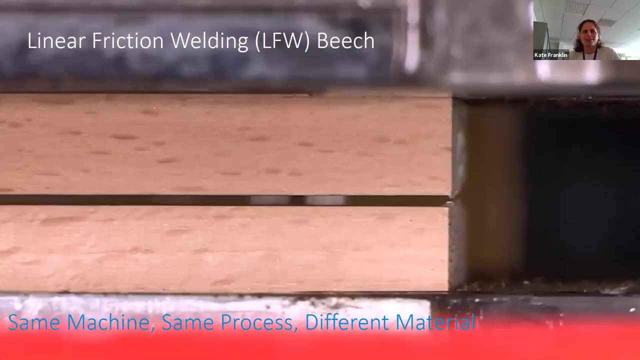 So the part at the end isn't exactly the best, But it is in the perfect position that you would want it to be, And you can see at the end of the process there is some smoke but no fire, And so we think we've proved the proverb wrong. 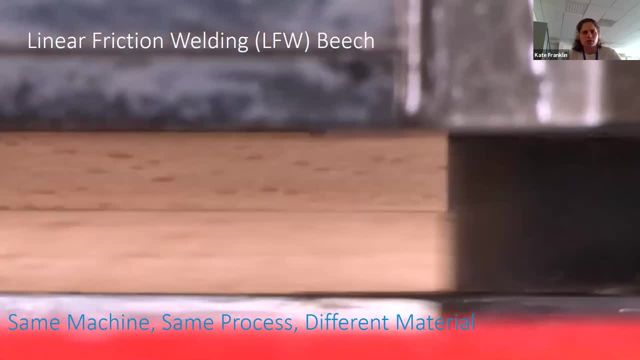 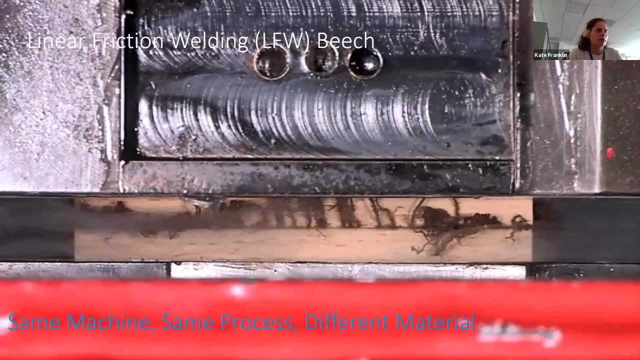 We've been really impressed with the initial results. It's produced a very strong join and, as your Darcia will explain a little bit more about the strength and the surface. And as your Darcia will explain a little bit more about the strength and the surface. 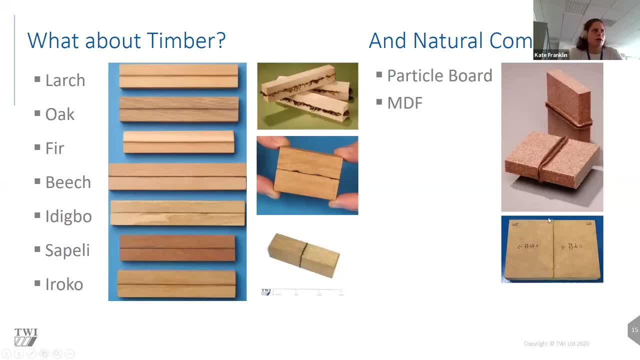 okay, so what about other materials? so we've not just welded beech, we've investigated other different species of wood and wood composites, including mdf and particle board, and i actually have some examples on my desk. so here is particle board now. i'm aware that that is. 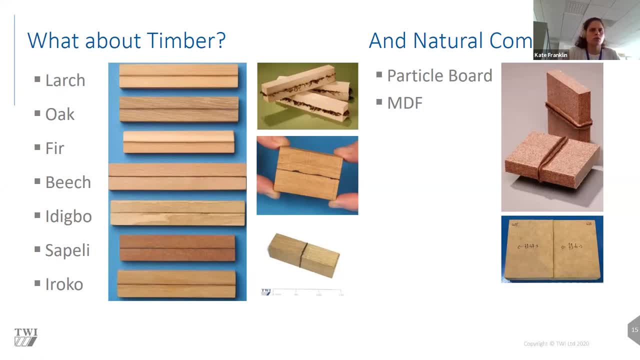 um got a high polymer content, so, um, that welds a lot more similar to other polymers and metallic materials. we've also- we've also got an example here of oak. now this is, i think, a hundred years old oak, i'm told, and on this part you can actually see the damage here. i don't know if 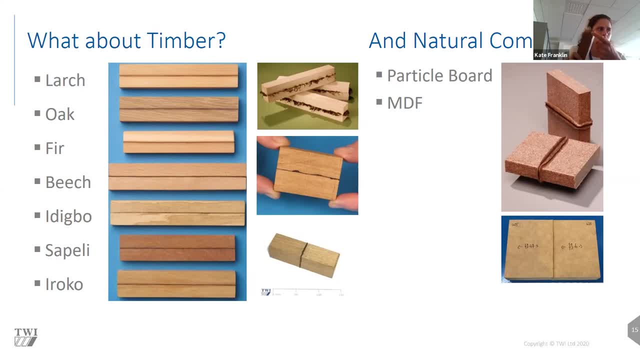 you can see me on on the screen or just the the presentation, but there's damage to the part of the wood, so i'm not sure if you can see it, but there's damage to the part of the part of the wood, so i'm not sure if you can see it, but there's damage to the part of the. 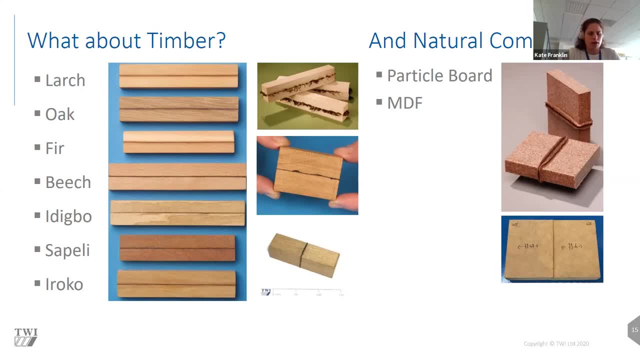 where we've tried to pull the joint apart and and it's failed in the fixture rather than in the joint itself. okay, so just to note that some examples shown here and some examples that you may find if you search for joining of wood in in literature, and they tend to use a different. 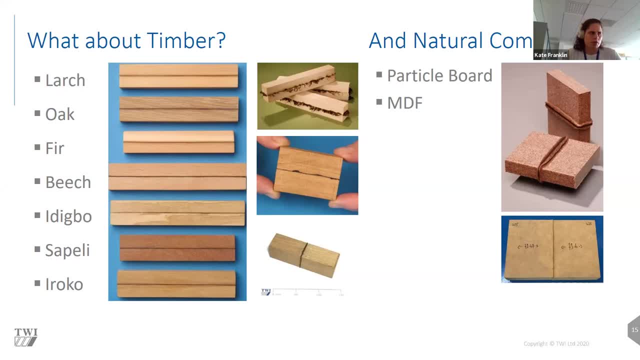 frequency domain, and so you might use vibration friction welding rather than linear friction welding, and we've had improved results using linear friction welding. so far, we've mostly looked at hard wood and produced great results. we don't currently know why these parts are joining so well, and that's why we're working with cambridge university to investigate the mechanisms at play. 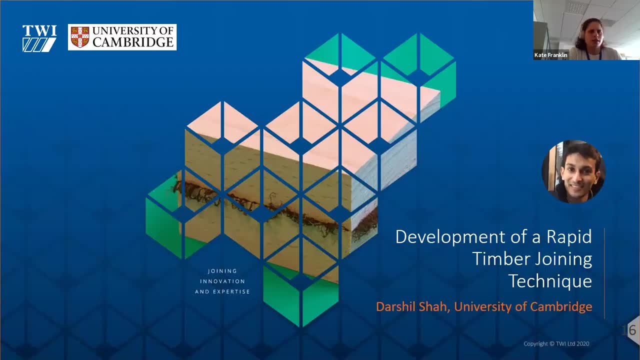 so that is where i'd like to pass you over to dr arshall shaw. thank you, kate. thank you, nick. um, yes, it's been a fantastic journey working with the twi. they are clearly the experts on this manufacturing process. uh, linear friction welding that we are using. 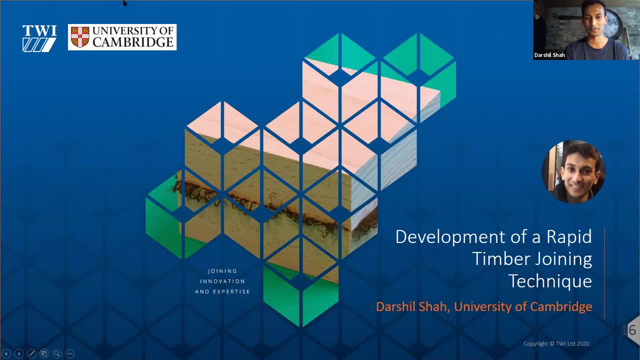 um. our expertise at the department of architecture in the center for natural material innovation lies with the material engineering department of architecture and the department of natural materials, in this case particularly timber. so i'll start off by introducing our center, but do remind me that i also have some samples to show, if i forget. 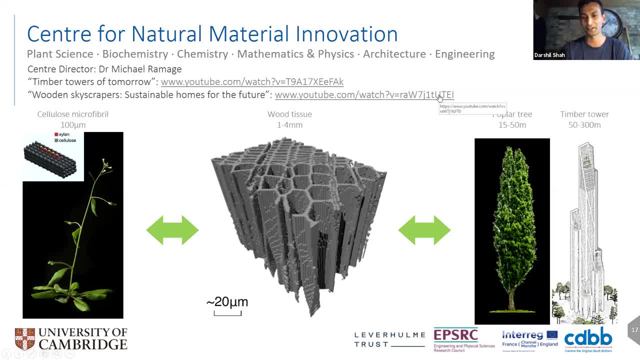 so i'm at the center for natural material innovation, where we work with a range of plant-based materials, primarily for the construction and building sector, but also for a range of other engineering applications, such as looking at the natural fibers- uh like flax, linen and hemp- for uh, wind energy or aerospace and automotive. 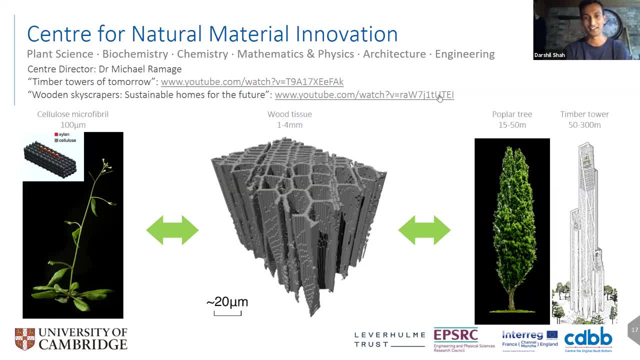 components. for example, at the back over there, uh, there is a automotive panel part um that is made from flax composites. um, but timber and bamboo are materials that we use for more mass scale applications, particularly in the building and construction industry. um. our center is multidisciplinary. we work across a range of departments, from plant sciences and biochemistry. 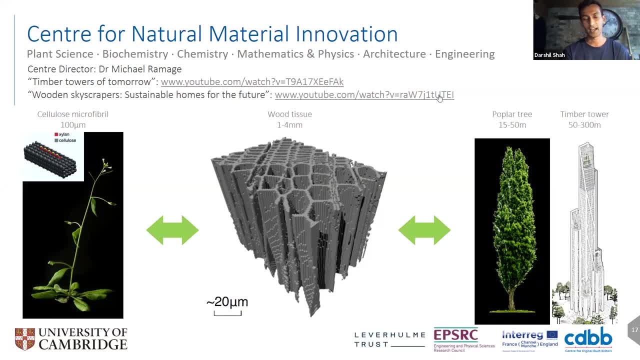 where our colleagues and scientists work at the very small scale. so looking at how cellulose the basic building block of timber forms and how it arranges with the other cell wall polymers and how wood gets its properties. we also work at the tissue scale with colleagues in chemistry and mathematics and physics, for example, looking at how 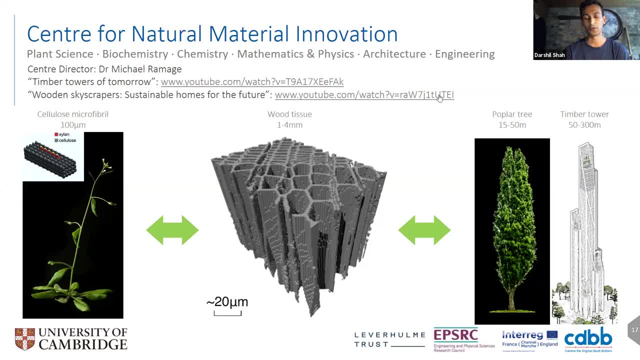 polymers may be impregnated into wood to enhance the mechanical performance and the durability of wood, and this is both to look at the applications of timbers and engineered timbers and building and construction, but also to explore how we may be able to preserve national treasures like the mary. 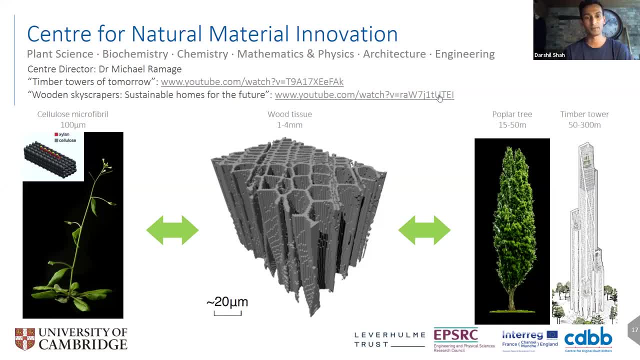 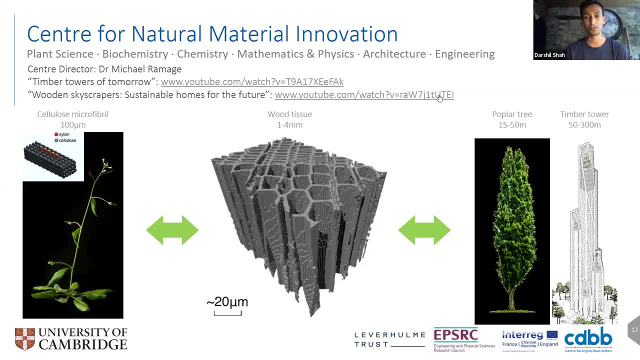 impregnating them with polymers can introduce some durability as well as dimensional stability. and then we also work at the macro scale, particularly with engineered timbers, to look at the design of the wood and construction of buildings and schools and other structures in which we need to live, work and be treated in. for example, There are a couple of YouTube. 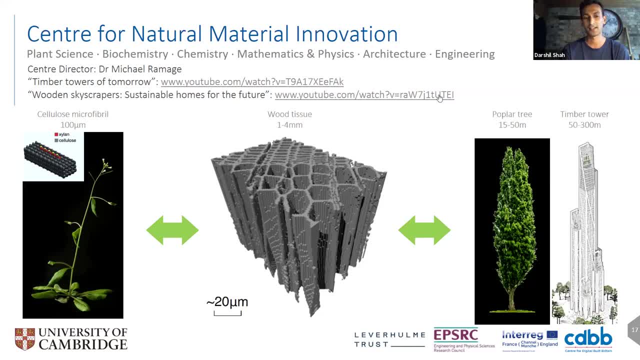 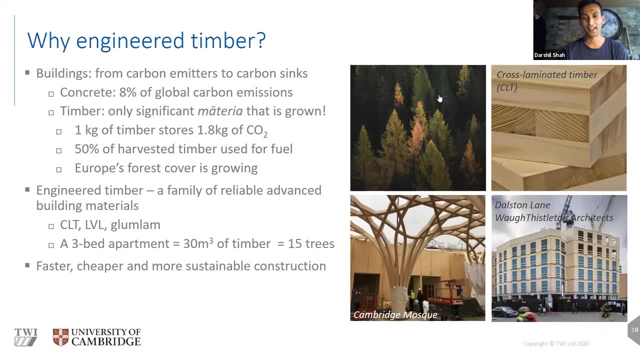 videos links up there which you can look at if you want to know a bit more about our range of research. The wood welding work that we have done with the TWI started off a couple of years ago now and my colleagues Dr Eleni Tumpanaki, 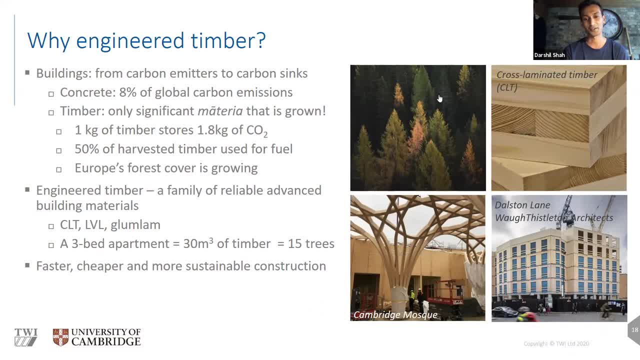 who's now a lecturer at the University of Bristol, as well as Dr Tom Reynolds, who is now a lecturer at the University of Edinburgh, are also involved in this project. Our primary interests lie with engineered timber, and this is not your ordinary timber that you can get from BNQ, for example. It's structural. 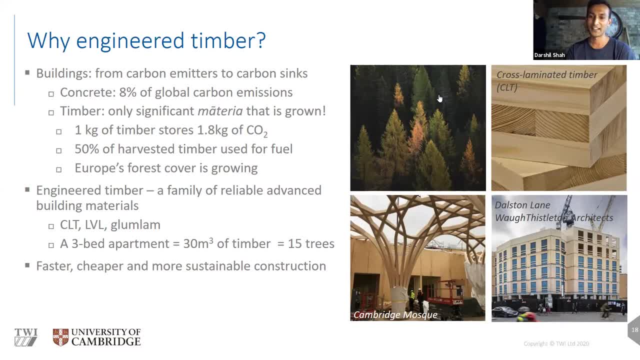 timber that you can get- from an seated house, for example- It's just that you can get- would use for mass construction. An example of an engineered timber is, for example, cross-laminated timber, in which you have- if you can see a sample over here in the right light- you have a number. 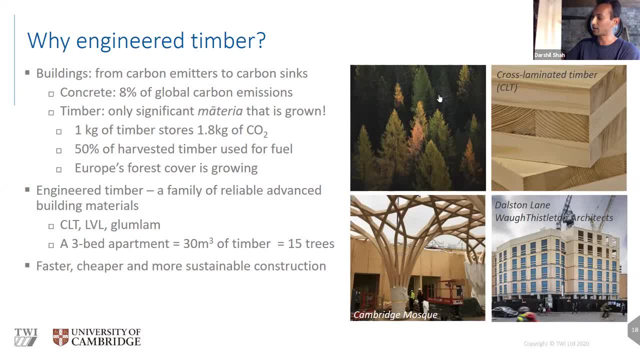 of layers of sawn wood that are glued together at 0-90 degrees and you can produce these at large scale. and there are a couple of companies, firms, large firms that we work and collaborate with, such as Storer Enzo, who produce CLT panels several meters long for use in floors as walls. 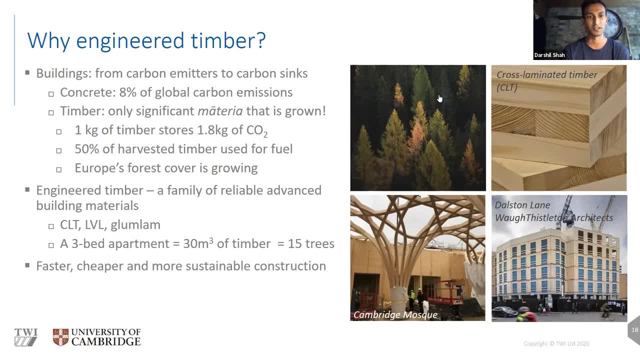 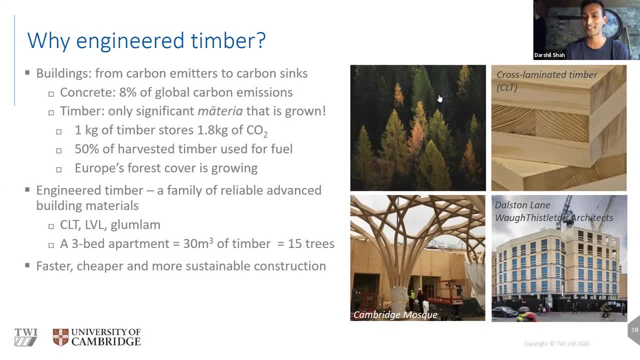 complex. they're quite complex. they're quite complex. But we also need to be aware that buildings can be carbon sinks rather than just carbon emitters. The building and construction industry, not only in the UK but also globally, is responsible for 30-40% of global carbon emissions. 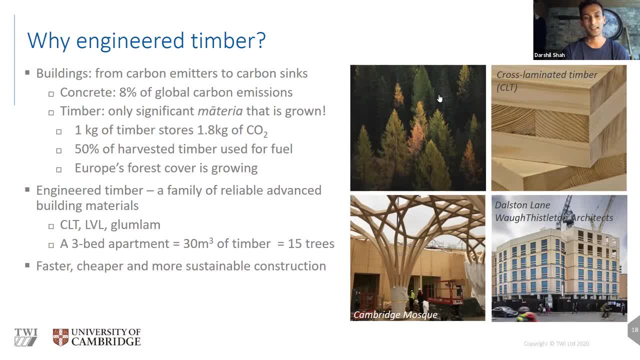 as well as energy consumption, as well as solid waste, actually- And concrete is one of the biggest culprits for this- and we should be using plant-based materials like timber, which are the only significant materials, and we should be using them in other employment projects and that's. 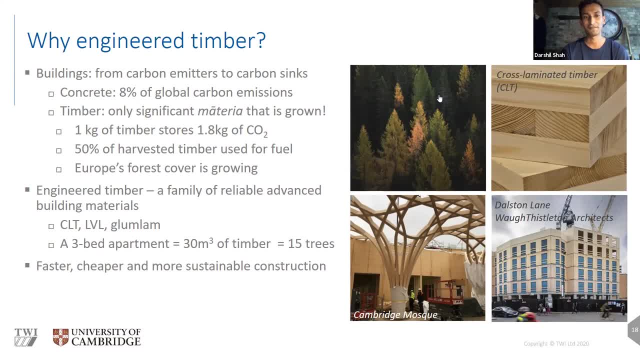 material that are grown and are renewable. In fact, the word material itself derives from the Latin materia, which means the trunk of a tree, And this is a material that we have been working with for thousands of years, and still we are learning new technologies with it, Each kilogram. 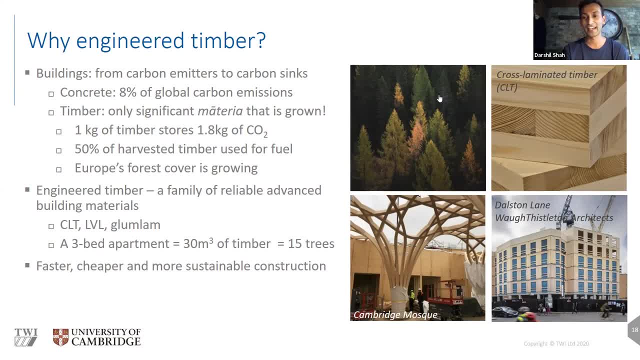 of timber stores 1.6 to 1.8 kilograms of carbon dioxide and hence goes on to show again the opportunity to use it for long-span applications or long-term applications, particularly because 50% of globally harvested timbers are used straight away for fuel wood. 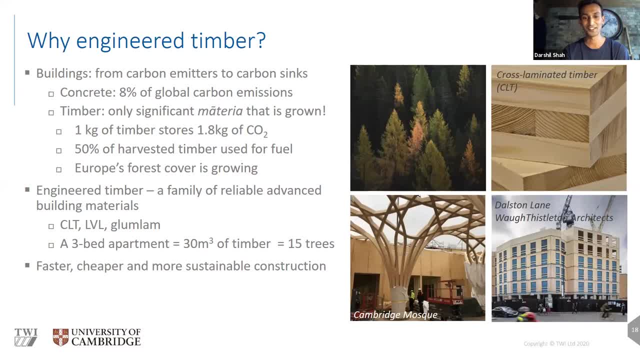 And rather than burning this valuable resource for energy recovery, we should be using it for longer-term applications, longer lifespan applications, and then thinking of other alternative end-of-life routes. Deforestation is a concern, but we should know that, for example, Europe's forest cover is growing and a lot of other. 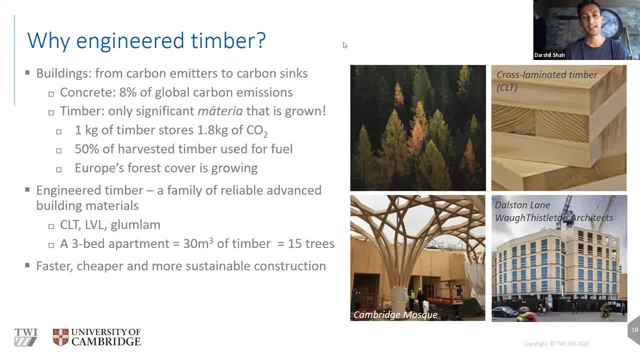 continents are afforesting quite rapidly. Biodiversity and managing the biodiversity in our forest cover is a concern, And we should know that, for example, Europe's forest cover is growing and a lot of other continents are afforesting quite rapidly. Biodiversity and managing 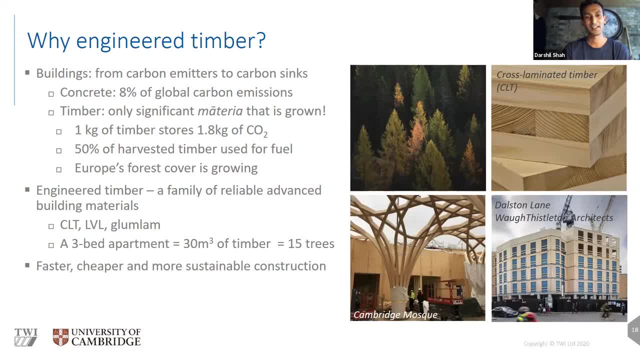 forests and the numbers of our forest area, as well as how much valuable resource we can get from it, is important, But nonetheless engineered timbers like CLT, LVL, laminated veneer lumber, in which we have thin veneers of timbers that are glued together all in the same grain direction to 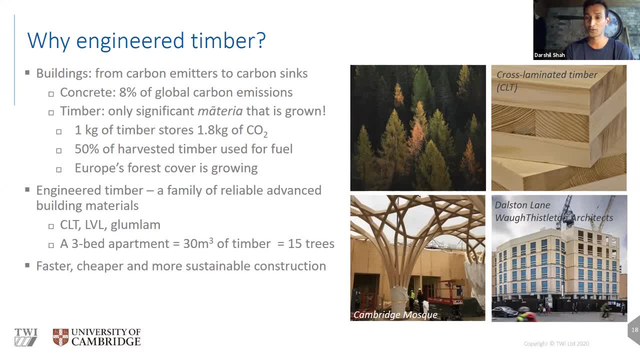 provide substantial strength are also useful in such building applications. A three-bedroom apartment that were to be made from engineered timber would require 15 trees. Now, if you think in comparison, in the UK, for example, an average person uses about eight to 10 trees per year. 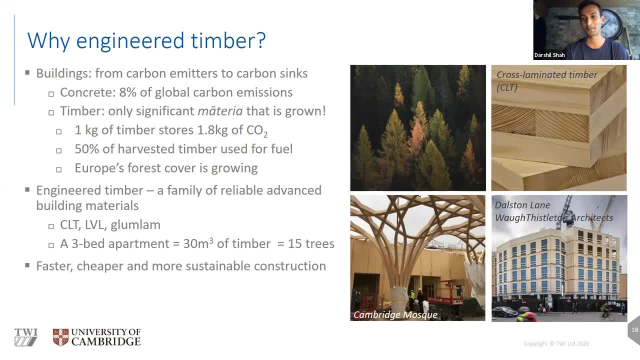 just for paper, And these three-bedroom apartments would be designed for at least 50 to 70 years and probably survive even longer. So there is a lot of value for us to get from using these plant-based materials for the construction sector, not only for sustainability. 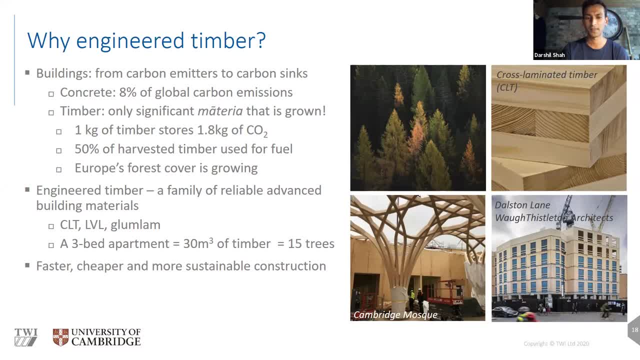 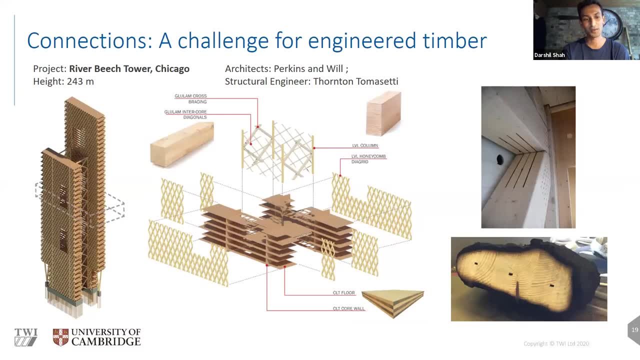 but also for rapid construction and cheaper construction. Moving on from this, there are a number of challenges that we need to overcome if we are to explore the construction of timber, especially innovating with it, for example, to create taller buildings. We, for example, 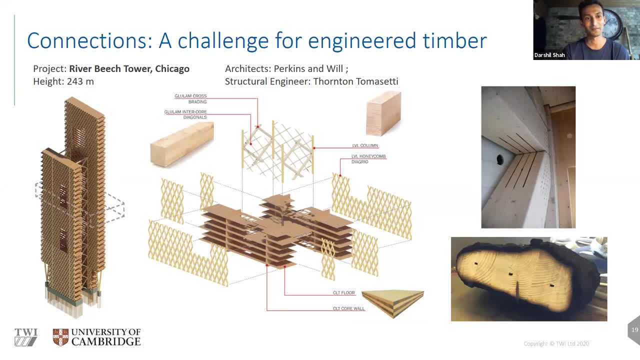 have worked with a number of engineering and architectural firms, such as this concept design with Perkins and Will and Thornton-Thomasetti, the River Beach Tower in Chicago, which is designed to be 240 meters tall and it uses a combination of glulam LVL. 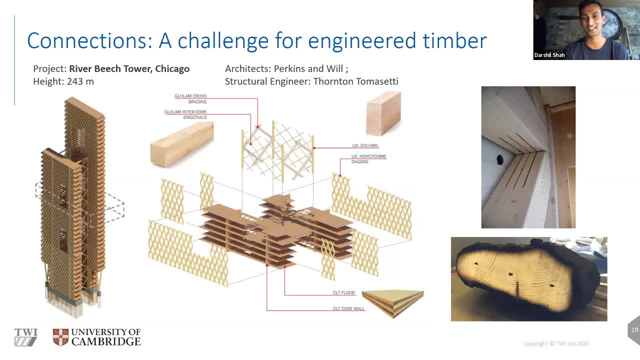 and CLT. One of the challenges with these sorts of designs is the connections, because the connections, how different components- for example, walls and floors- how they connect to each other, are the weak point of the design. So, for example, if you have a building that has a lot of 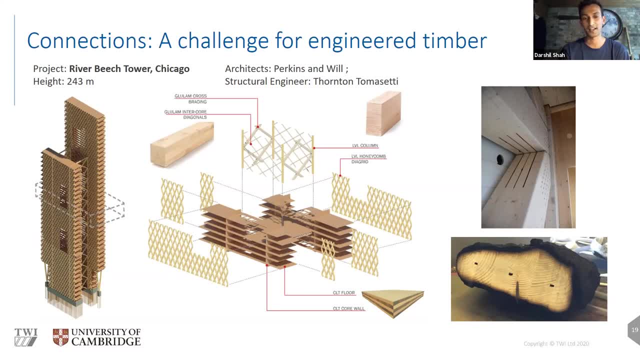 joints and therefore we need to either understand how we can strengthen these or make them more durable. Often, these joints are using metallic fasteners, for example, or using polymer adhesives or composites, for example glued-in-rod CFRP or GFRP materials. The other challenge is also fire. 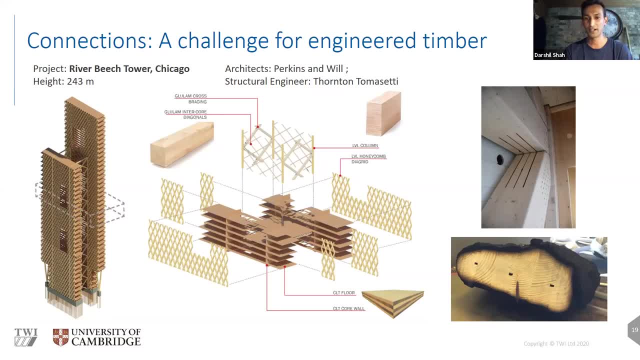 and although wood burns at a known rate and the charring rate is constant, what tends to happen in an engineered material such as CLT is that, once the temperature has, once the fire has progressed into the material and it reaches a glue line, the layer delaminates and fresh wood is exposed. 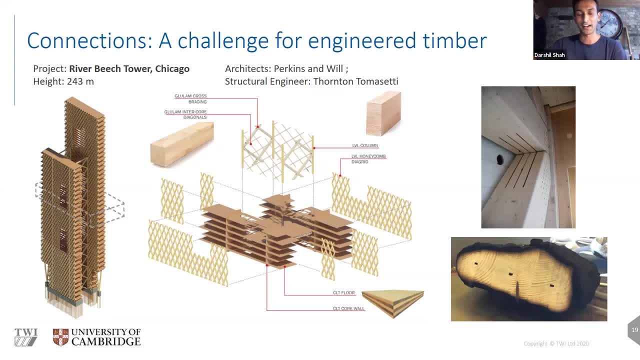 and that leads to continued progress of the fire. And therefore, if we were to think of other methods of fire, we would have to think of a different method of fire, and that would be the first one. The second one is that we would have to think of other methods of joining timbers more efficiently. 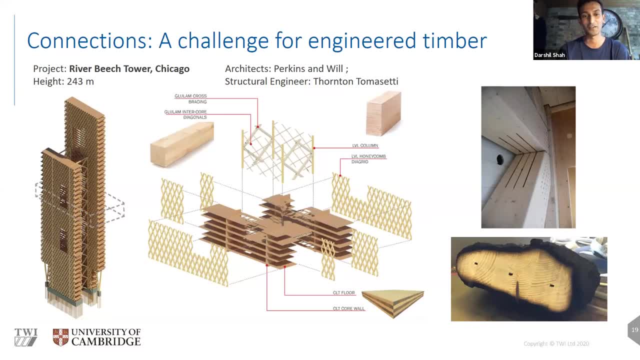 that can help take this material even further into our homes, for furniture, but also for the building and construction sector, And therefore we have been working with TWI on this fantastic technology of wood welding, And in the next slide there are some initial 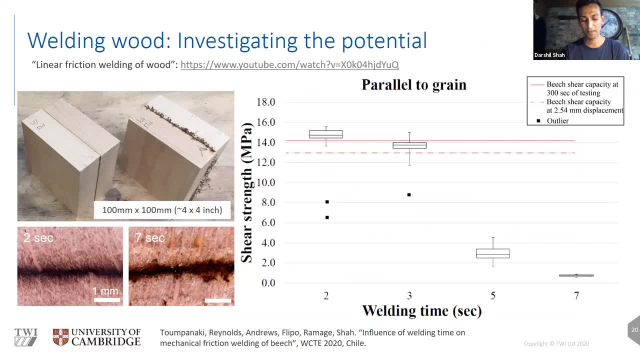 results that we have obtained. So, as Kate mentioned to you, TWI themselves have tested a range of different timbers, both hardwoods and softwoods, as well as wood composites like MDF We particularly have gone on to look at in a 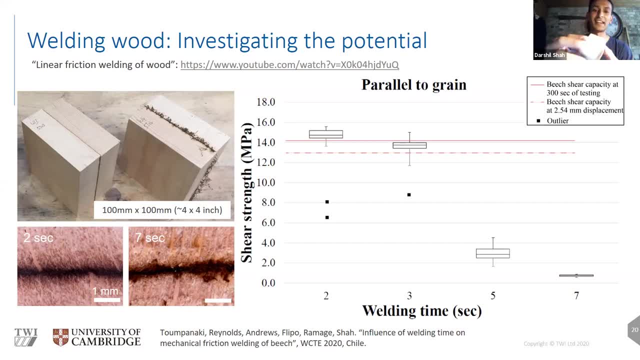 bit more detail into beech. So this is an example of a welded wood sample. and then, if you were to break it in shear mode, you can see what the failure surface looks like. So there is some substrate. and then you can see what the failure surface looks like. So there is some substrate. 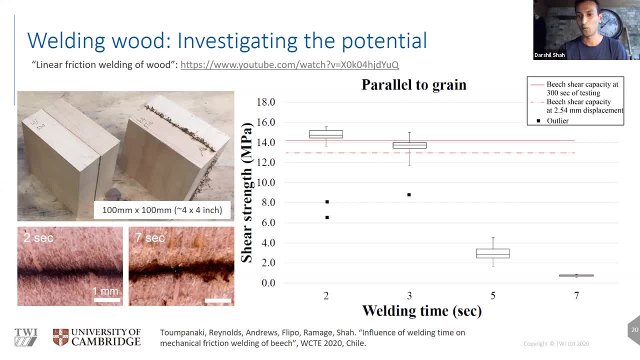 failure as well as some failure along the weld line in the material. So it's a mixed bond failure which can give quite high shear strengths. Many of these were tested at the same frequency of 75 hertz and, as Kate again mentioned, this is in the linear friction. 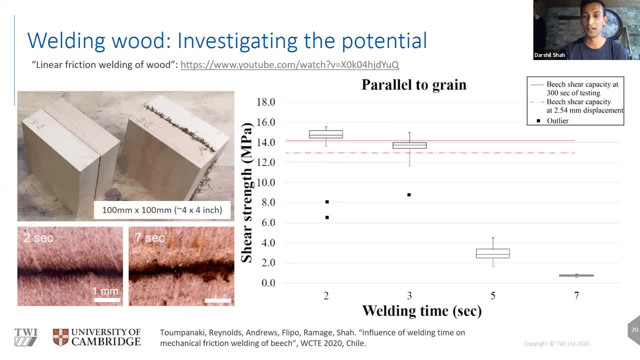 welding frequency domain. Much of the literature studies have primarily used vibration welding at much higher frequencies, Sometimes exceeding 150, 200 hertz. What we have done is look at the effect of welding time on the shear strengths of the materials of the joint. Anecdotally, we observed that weld times of one 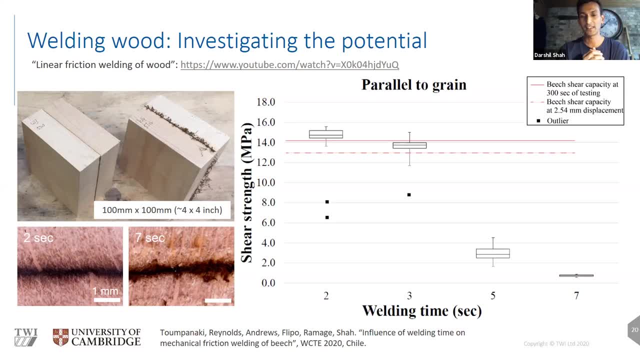 second didn't form a bond, and we think this is because the heat generated during the friction process wasn't enough to initiate that bond. and that is primarily because one of the cell wall polymers in wood is lignin and that is a thermoplastic and it starts to melt and flow. 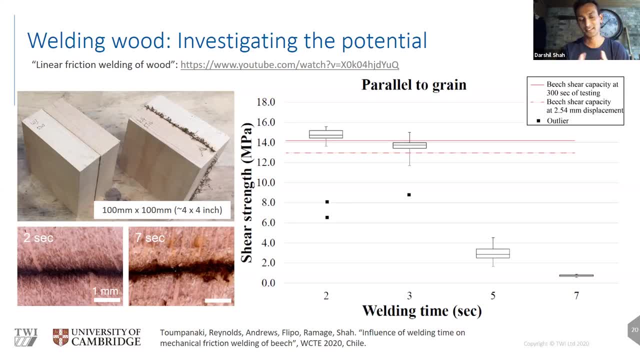 after a certain temperature and a weld time of one second would not have possibly reached that temperature. However, weld times of two and three seconds give a lot of heat, So this is a really high shear strength values in the range between 13 to 15 megapascals, and the very exciting 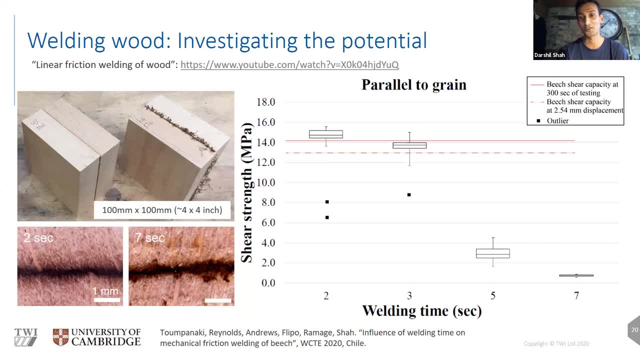 thing is that this exceeds, or is at least comparable to the shear capacity of beech itself. So the bond, the weld that we create is stronger than the wood itself, which is a dream for any material scientist. At higher weld times of five and seven seconds, we see a dramatic increase in. 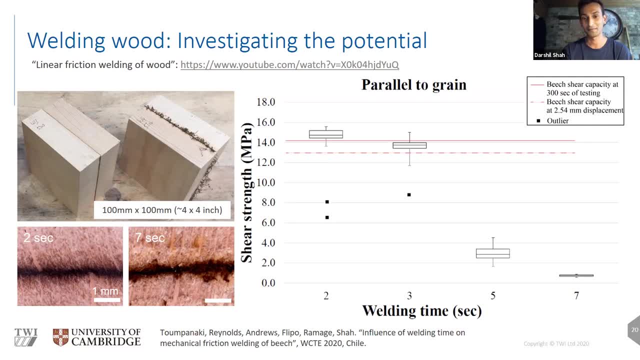 the shear strength of less than five megapascals. And this may be because at higher weld times the heat generated is the temperature reached is much higher, leading to degradation, probably thermal and mechanical, of lignin and other cell wall polymers and therefore the weld. 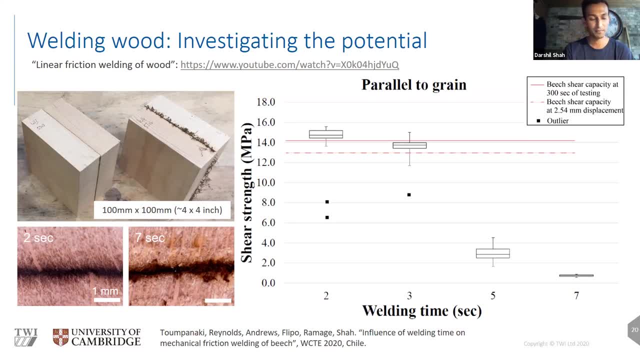 shear strength is much lower. We also see that the heat generated is much higher, and so the heat generated is much higher. We also see that the heat generated is much higher, and so the, based on our microscopy, results that, and there are a couple of micrographs on the slide over there. 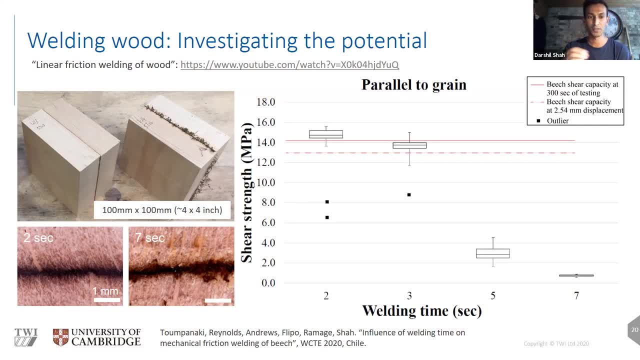 that higher weld times the weld line has much more porosity, and higher porosity often leads to has a detrimental effect on the shear strength. In the next slide we've also tried to compare some of our results with those in literature. 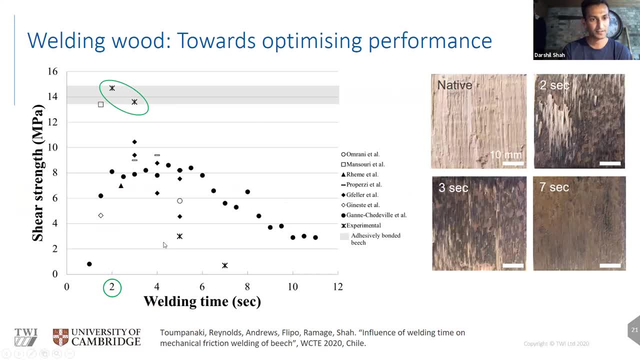 I move the slide. Perfect, Thanks, Kate. And as you can see, our results compare quite favorably in comparison to those in literature. Our weld, the weld times of two and three seconds, give a shear strength of 13 to 15 megapascals, and that is substantially higher than what has been reported. 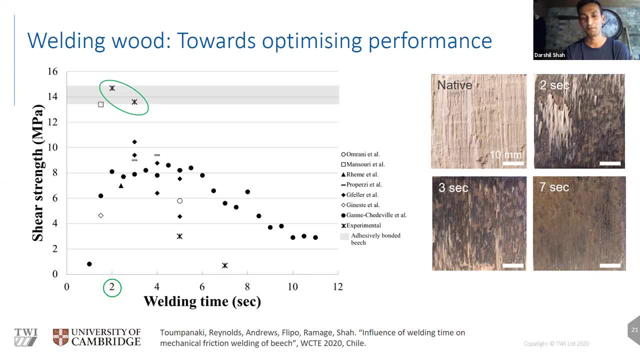 in literature And, as I mentioned, that's primarily because we have been applying this technique using linear friction welding rather than vibration friction welding, which has been primarily looked at in literature. But nonetheless, you tend to see this interesting profile of how weld time affects the shear strength in the bond line And weld time so far. 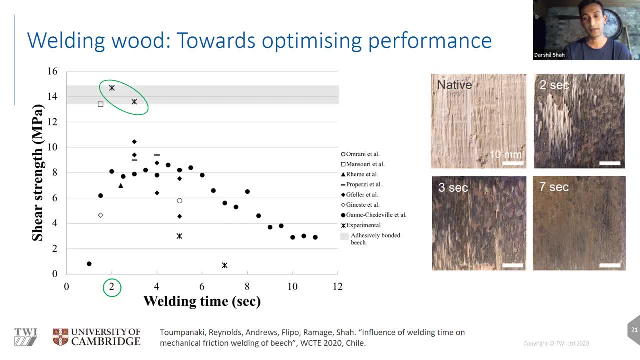 is the only parameter that we have changed, or much more systematically changed. There are lots of opportunities to not only change weld time, but also the pressure with which you're putting together the bead samples, for example, as well as the vibration amplitude and the frequency of vibration, And we'll be interested in looking at how all of these come. 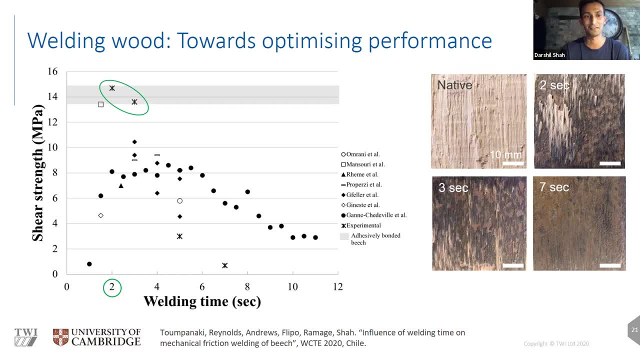 together and how they can be optimized to give possibly even higher shear strengths. Wouldn't that be amazing? There are some micrographs of failure surfaces. again You can see the different brittle and ductile failure surfaces. at higher weld times It's a very smooth and shiny surface. 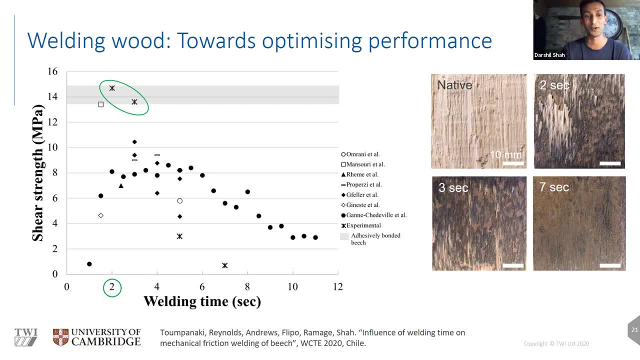 which is characteristic of the low shear strength, And whereas weld times of two and three seconds, you can see some substrate failure and lots of shear failure in the wood itself, And this is many times. these Kevin Fuller tutorials are not the only pieces of evidence. 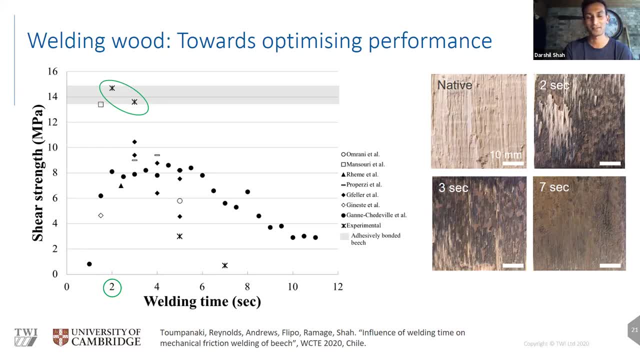 but specifically at Capac Anneli, Chapter 3, Home API. Here we can get more context on wood breaking and how wood ihes 256 cayenne sucedège and that chilling rate is the structure of the bond line and how theciu modelling some numerical measurements on them. 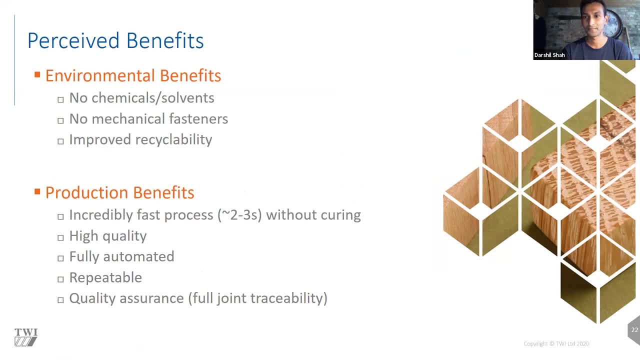 old 서, So we'll have to wait a little. I believe there's probably some congregation here, I think. right, Betty, Here one with the prejudices, this one for sure. cough, Here one with the prejudices, this one for sure. 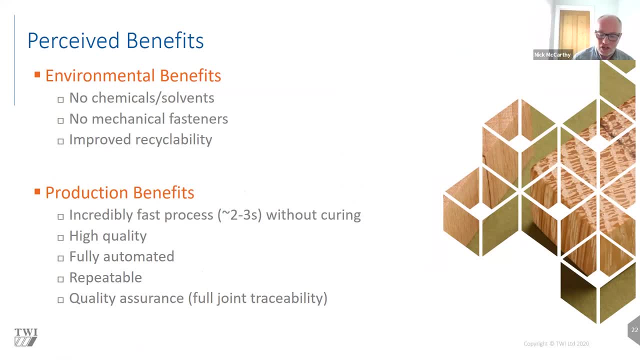 Rachelesian, Over here you can see the details of the load dynamic, faudragen, 매 or zestar et cetera phone. I'm pleased to say Thank you, Darshil, Thank you Kate. Fascinating presentations. 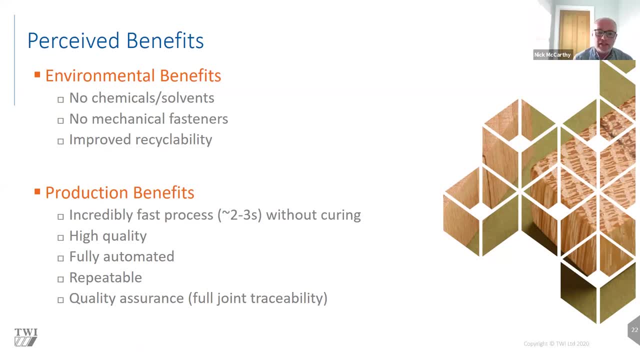 really informative And hopefully the people on the webinar can start to really see the potential benefits And, I think, more importantly as well, that the potential applications that we could aim for with these processes, on this process it's, it's something we're very 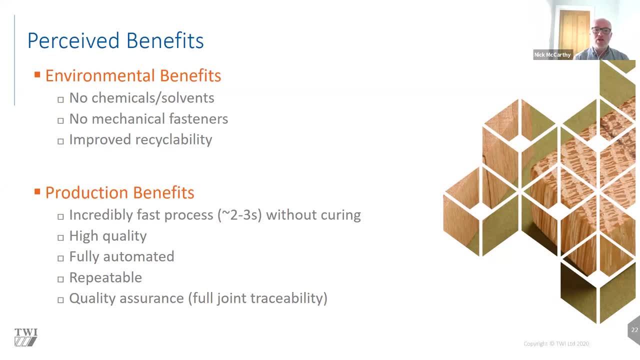 very excited about at TWI. I mean really. Darshil's touched upon some environmental benefits there that we've highlighted: Production benefits. you know, as Kate has suggested, potentially an incredibly fast process. you know the cycle time of the bond is two to three. 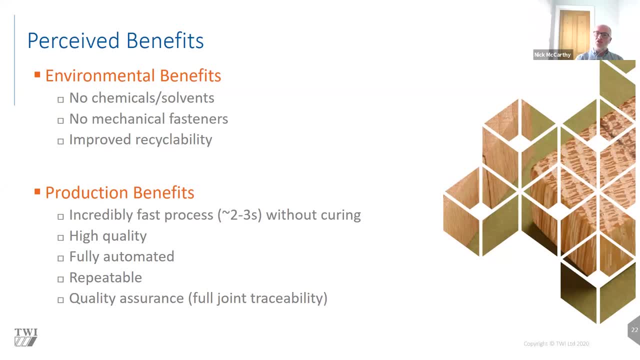 seconds And, as we can see from Darshil's slides, we've seen very, very promising results with with fast cycle times. You know the process has the potential to be fully automated. You know we're not dealing with any curing times or anything like that. It is a very, very repeatable. 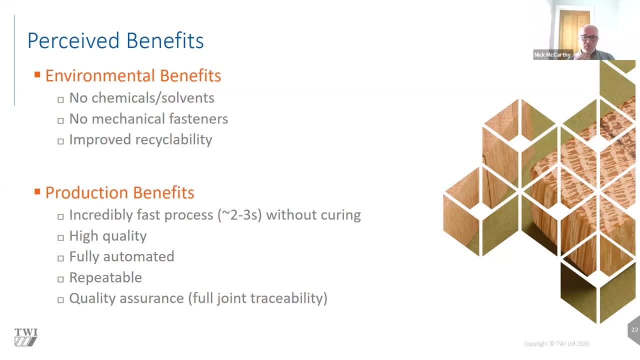 process And we know that because of the. you know, as we said at the beginning, it is an established process, It's a mature process And, as Kate highlighted it's it's used in very, very safe to critical applications. 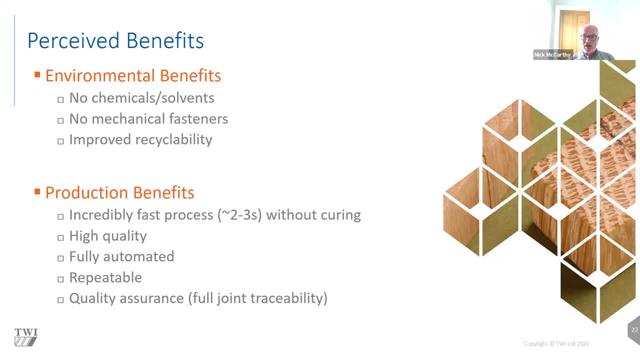 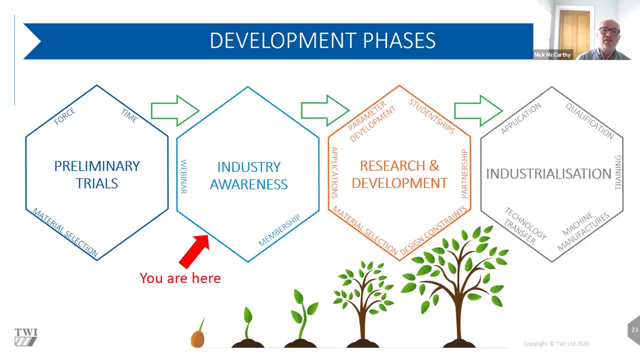 19, 10, And now you're watching us how to will onto the next slide: 20, 21, 22, 23, 24, 25, 26, 27, 28, 29, 30, 31, 32, 36, 31, 32, 32. 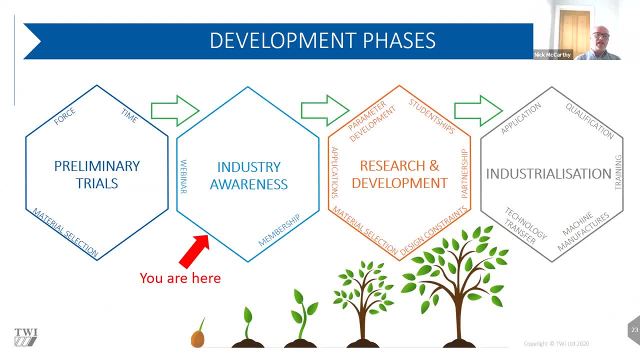 33, 33, 34 phases. i mean to be honest, the, the, the. we've done the effectively, the, the first, the first section there where we've done the preliminary trials, we, we've worked with some different materials, we've looked at the, the parameters of force and time, etc. and really this, this phase, is the industry. 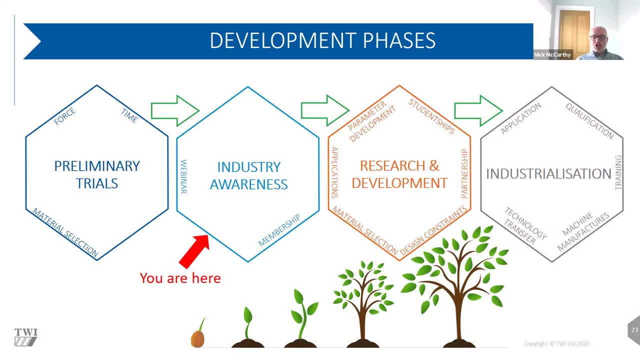 awareness phase. so this is really where we're, we're, we're pushing it out to industry and we're saying: you know, we, we have this technology, we have this, this, this idea that this could, could really be good in industry. what, what can you bring to us in terms of applications? so really, the next. 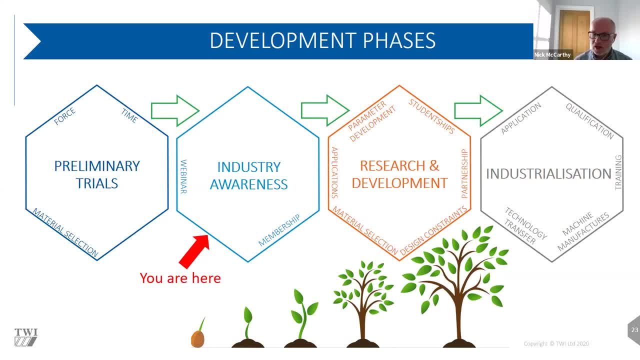 the next phase is this research and development phase is is is really where industry plays its part, where hopefully you can. you can see the potential in the process and you can come back to us with some. you can come back to us with some, you can come back to us with some. 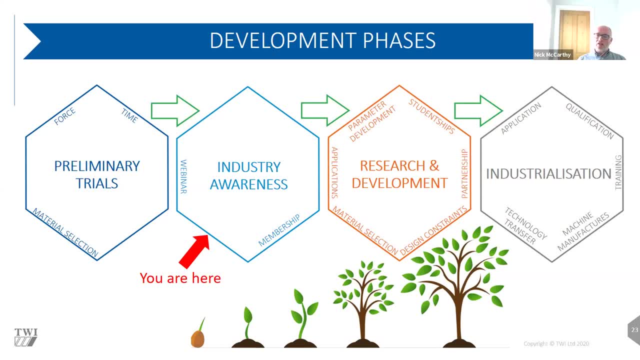 applications that we can. we can start to look at. we can, we can tell you whether we think it's a viable application and then we can. we can obviously look at partnering with you and moving the process forward, um and eventually that hopefully, if everything is successful, um it leads to. 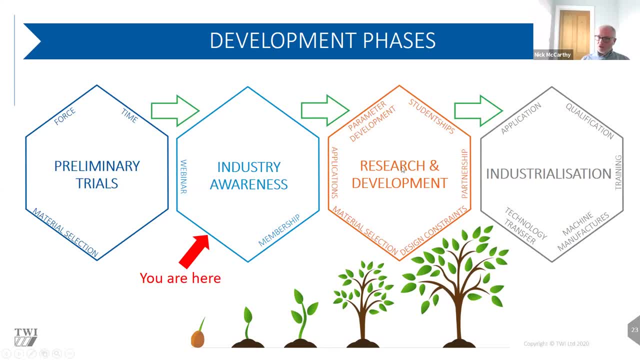 industrialization, um, and again, as i touched upon in the beginning and i believe, in fact, on this webinar today, i think there will be some, um, some of our members that are, in fact, machinery manufacturers. so you know, we are confident if we find a, an application, and the process is. 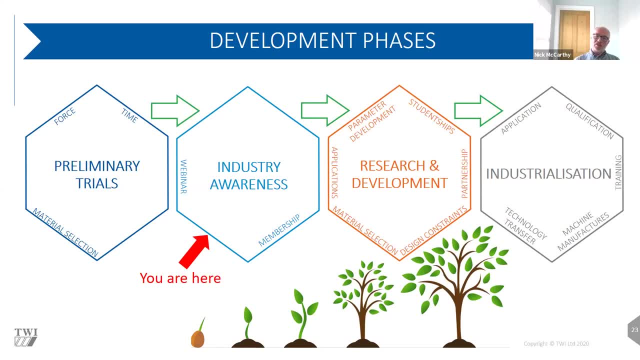 right for the application that we can then also help with the technology transfer moving you into industrialization, into to having a machine and and and carrying out this while being yourself. thank you, kate nick. may i also mention that, yes, we also have studentships. uh, twi supporting two. 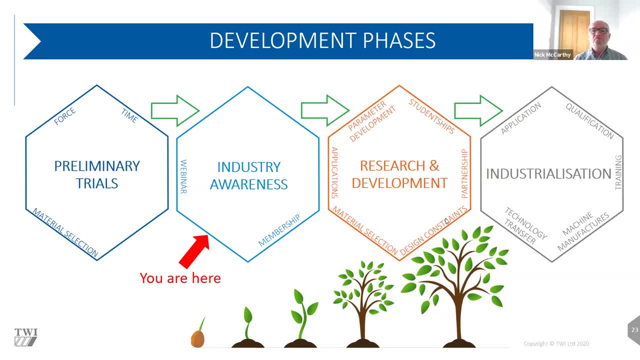 students at the university, and we have a lot of students at the university and we have a lot of university of cambridge, yeah- who will be working on an year-long project on wood welding and looking at, uh, a range of different types of woods, for example. thank you, narshall. yeah, much appreciated. 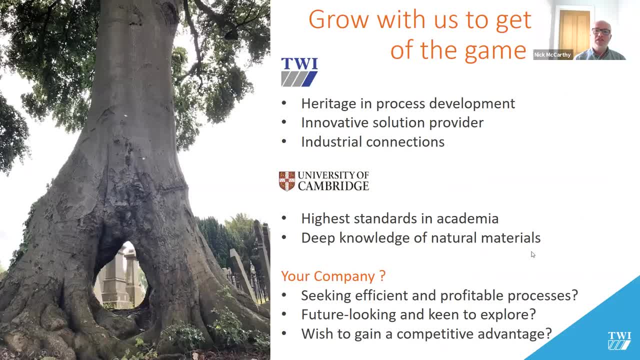 that's, that's, that's good thanks, kate. um. so yeah, to summarize, um, you know, hopefully, um we've illustrated that the twi have this heritage in in looking at processes, in developing processes, in working with our members to hopefully um take ideas from, from conception, right the way. 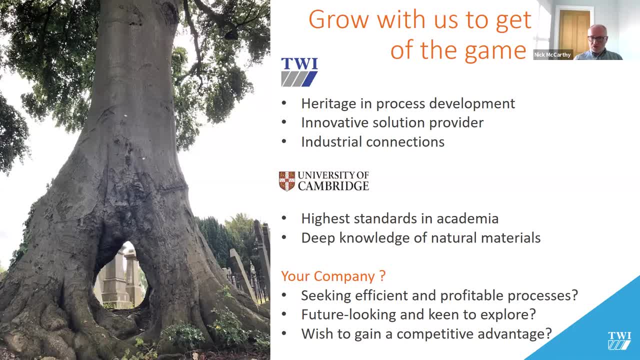 through to, to to, from inception, right the way through to to, uh, a manufactured product. um, you know, we, we, we, we like to say that we, we are, we know the materials, we know the joining processes and hopefully we can then help you, uh, adopt those joining processes. um, i think it's been. 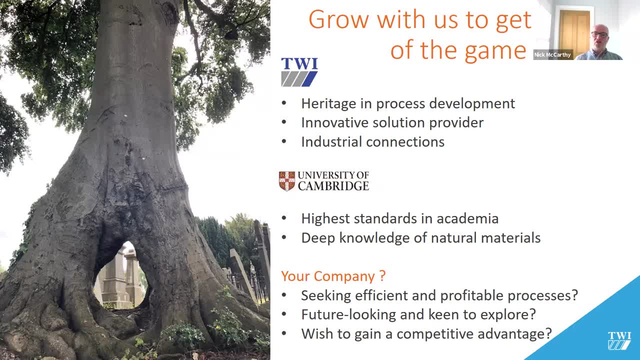 a pleasure to work with darshall, um and the university of cambridge on this, um. i think everybody's aware that they have, as it says, the higher standards in academia. um, and and darshall and his team obviously have also a deep knowledge of the of the natural materials as well, so thank. 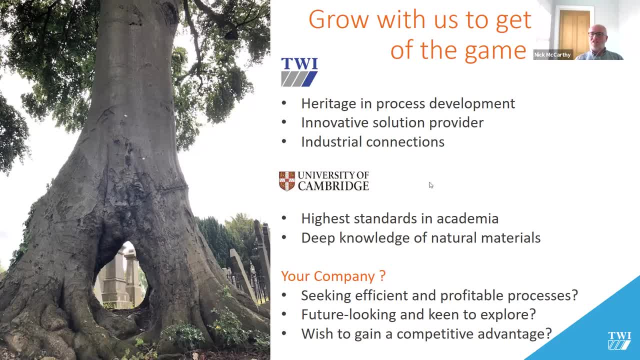 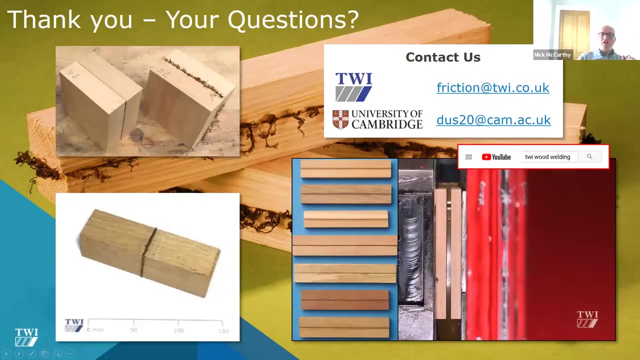 you very much for your participation in this and, uh, it's, it's, it's very good to work with you. um, so what we'd like to do is is: um, we've got quite a few questions. i think, um, sorry, kate, you can go back to that other side. that would be great. um, so we've got quite a few. 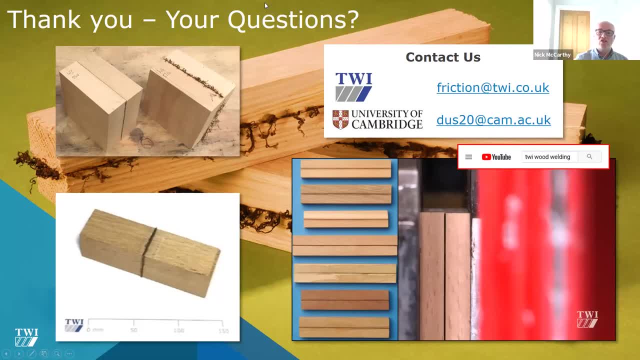 questions that have come in. um, and i'm gonna take a look at a few of those questions. um, here. um, we've a limited amount of time, um, so, as i said at the beginning, um, what, what i would, what i would suggest, is: um, we'll, we'll look at it, we'll address a few of the questions, but rest assured we've logged all. 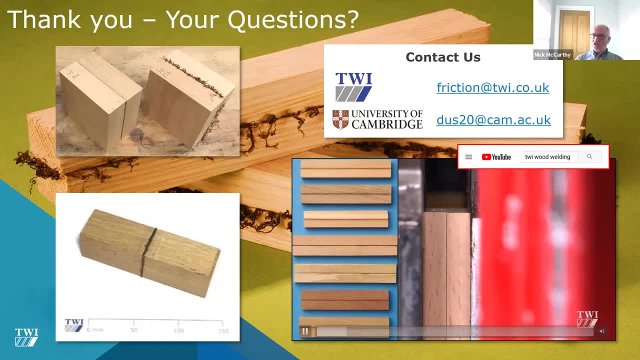 the questions. we have your contact details from from your registration and we will get back to you. we will get back to you with that as well. um, right, so just bear with me a minute. um, so, um, okay, so, um, i've got one here, which is: what is the influence of water content of the wood? 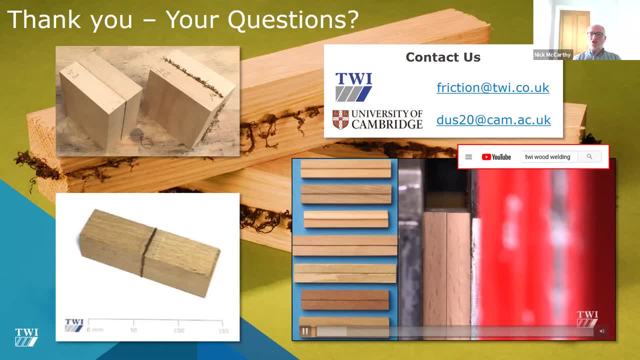 on the process. so, um, i don't know, darshall, do you would you like to? would you like to touch on that one? yeah, i think that's a great question. uh, the moisture content of the timber has an effect on the bond performance, both in terms of what the water moisture content is prior to the 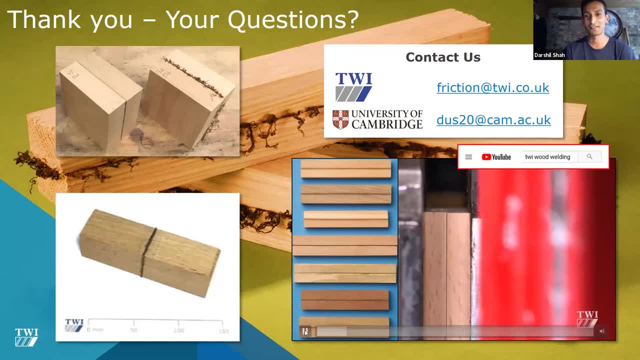 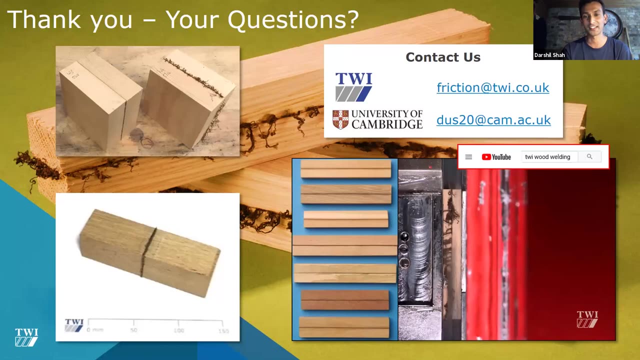 application process as well as, in service, the effects it may have on the actual bond. um some literature suggests, for example, that friction welding or vibration welding of drier wood results higher shear strengths. um so far, we have conducted our tests uh in a humidity controlled environment uh in which we know the moisture content, the equilibrium moisture content of our samples. 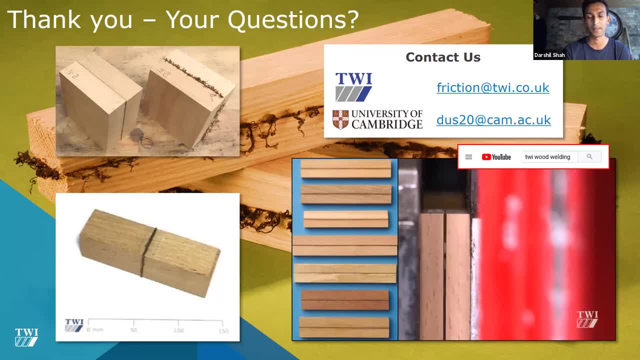 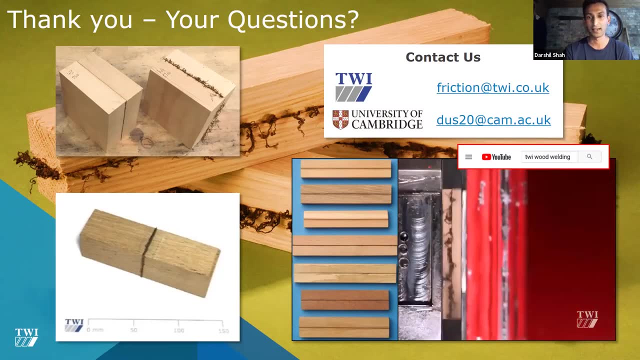 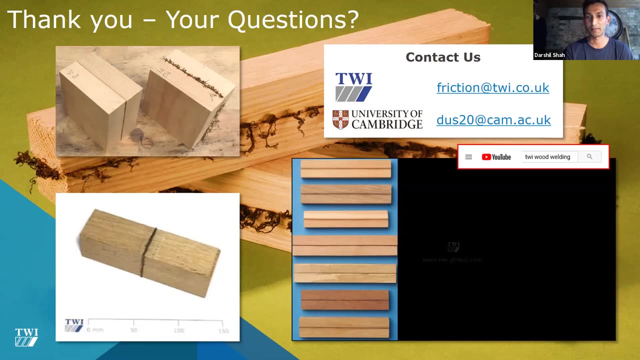 uh, it's in the range of 10 to 12 percent um, and that is often the equilibrium moisture content uh of uh engineered timbers, uh in the building sector, ranging between eight to twelve percent um. um, of course, uh because of the heat generated and the temperatures involved uh during even that. 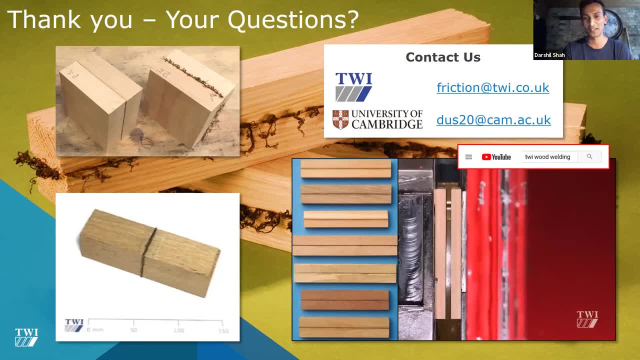 short time span in the heat affected zone, so to speak, or at the bond line, some of the moisture might uh evaporate or it may start to de-polymerize some of the uh polymers in the cell wall and therefore facilitate even the bond performance. um, but it is something we need to explore in a bit. 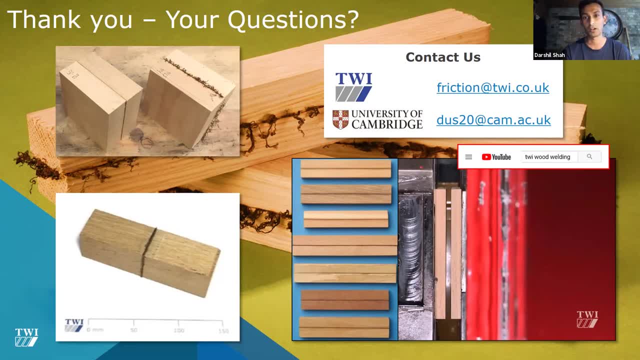 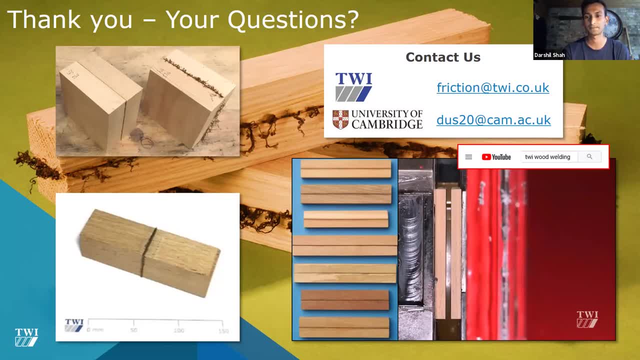 as well as looking at the aging performance of these bonds. fantastic, thank you, darshan. um, i've seen one uh question here which relates to: is there any sort of surface preparation required for the two pieces of wood to be welded? um, kate, would you like to? 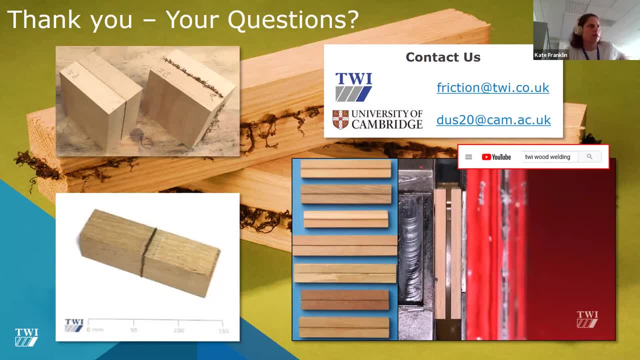 comment on that. yeah, so at the moment, um we we don't do any particularly special surface preparation. um, even when we're joining other materials like metal, um we'll, we'll machine that surface um, but there's not any edge preparation like there would be in a manual art welding process or 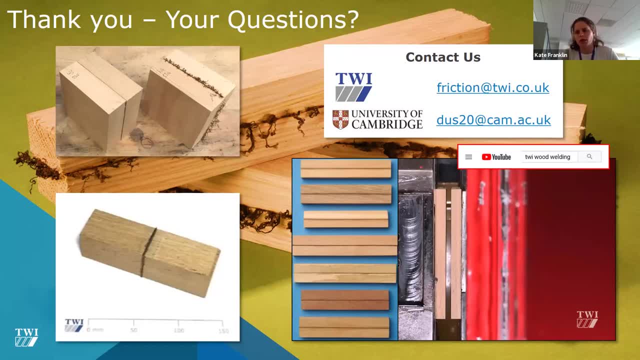 or another welding process. so at the moment where we've not done anything to the surface of the wood, we've literally just cut it um. but we are interested to look into um what a effect applying something like lignin to the surface might have on the characteristics of the 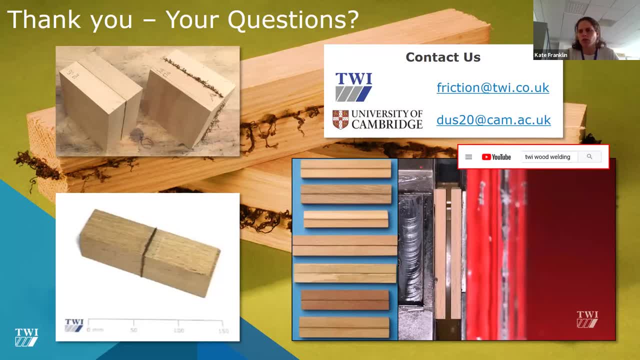 bond and, but at the moment, yeah, it's, it's literally just cut and and then joined together. great, okay, um, i've got another one here which i'm going to throw at you guys, which is: have there been any tests or results from softwoods like pine? 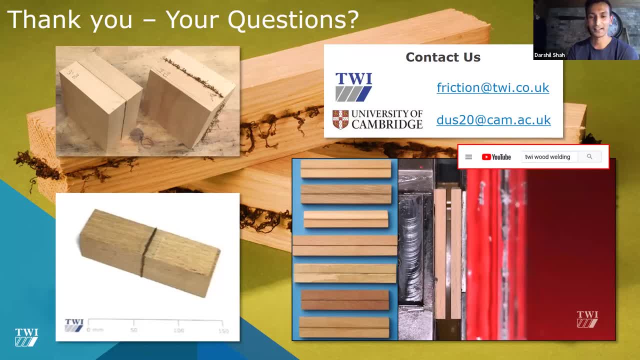 i think we'd throw that one probably over to darshan, have you? yes, yeah, i think. uh, twi have run some tests on softwoods, not in pine, but they have run on fur and large, i think. um, and we are still not entirely sure what makes this happen in the sense, even though there are a wide variety of species of trees, 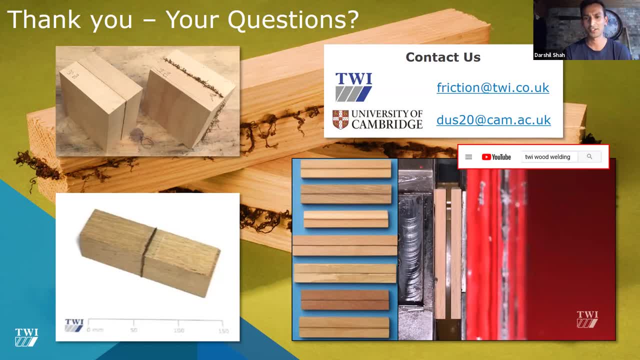 and each species would have a different combination of cell polymers, for example lignin content, and even the lignin is different in the different uh species, and therefore trying to understand, trying to better understand how biochemical composition relates to the bond performance is something we're interested in doing. 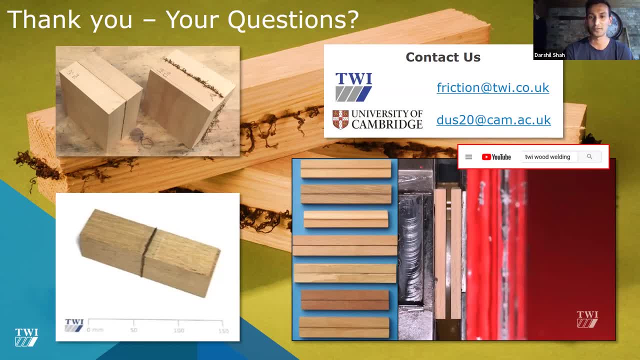 so, as part of the student ships, uh, the two students that will be working with twr and ourselves, we'll be looking at, for example, one uh softwood, uh spruce, for example, which is commonly used, uh for cross laminated timber, uh as well as beach, because we want to further this research. 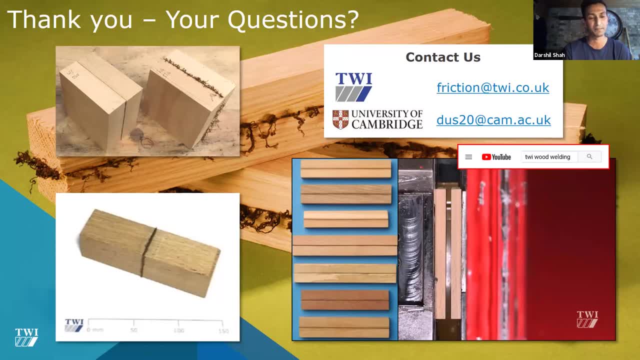 beach is also used in laminated veneer lumber in europe, for example. and we also want to look at bamboo. bamboo is a fascinating material that we and it is a grass which is not a wood actually- and trying to understand how the sugars as well as the starches and 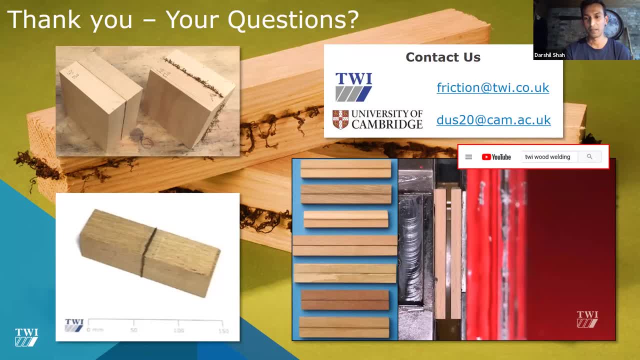 lignin influence. the bond performance would be interesting, uh, for us to know. fantastic, um, we've got a a great number of questions. i'm delighted to say i think we're we're we're running out of time on the webinar now as well, so we will be answering some of these. 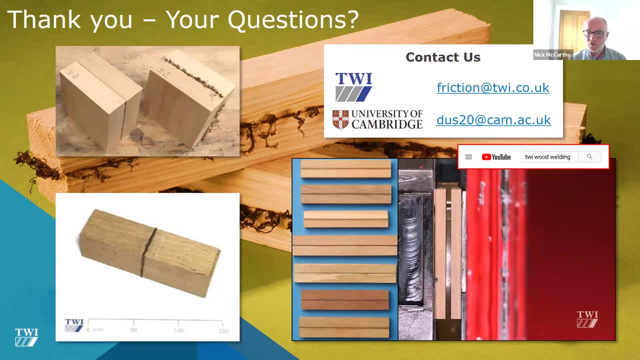 after the webinar. but rest assured, anything that's been raised in there we will be getting back to you. um, there's, i think there's one. one further question which i think is quite an interesting one is: can dissimilar types of of woods or timbers be joined? who wants to take that one? i guess i'll. 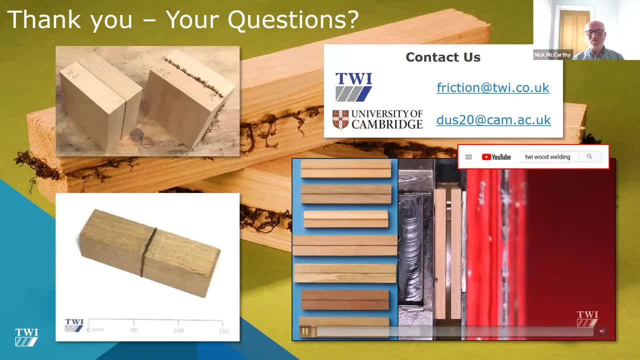 take that for now. so, um, again, it's not something that we've tried. at the minute we're still in initial um phases of testing and we'd love to get someone on board that wants to try to join dissimilar wood. um, it is a technique that's used to join dissimilar materials. 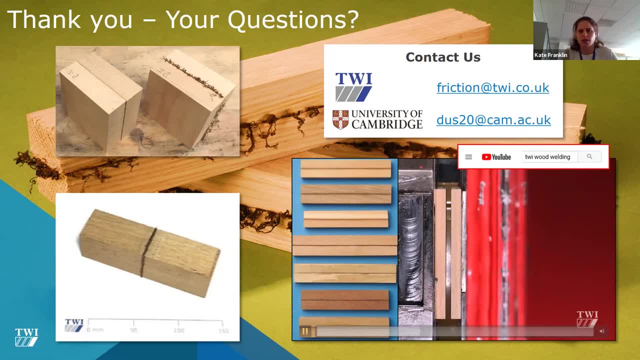 and it and it's known for being very good at that within the industry, and so it's often used for joining steel to aluminium, for instance, and we've also done some trials um join thermo plastics to composite materials and thermosets using a thermoplastic interlayer to 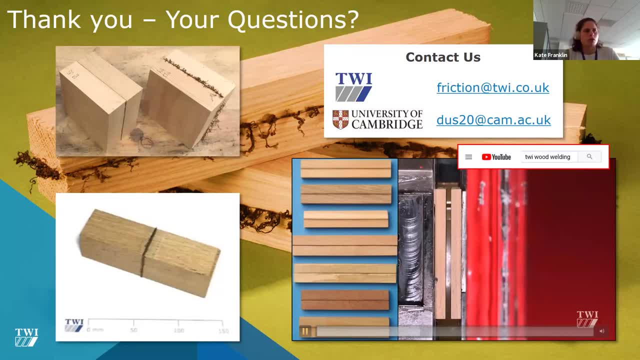 um composite materials, um. so we've tried it on um other materials using dissimilar things, and it's it's worked very well. it's it's known for working really well, but on wood we've. we haven't tried that yet, but we'd be really keen to give it a go if someone wanted to come on board. 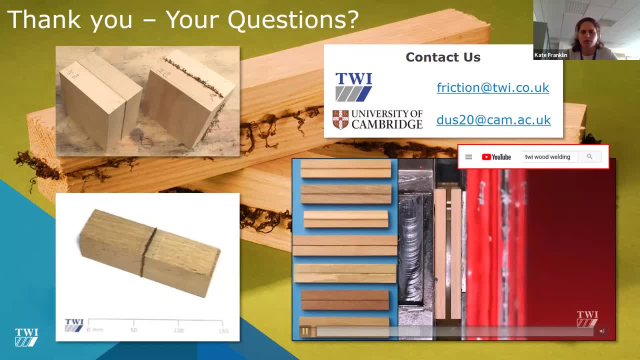 and try that with us. i don't know if, dasha, if you have any additional technical comments on that. no, i think that's entirely right. uh, it, it's quite. our hypothesis would be: yes, it should be able to, especially if you have one material that has, for example, 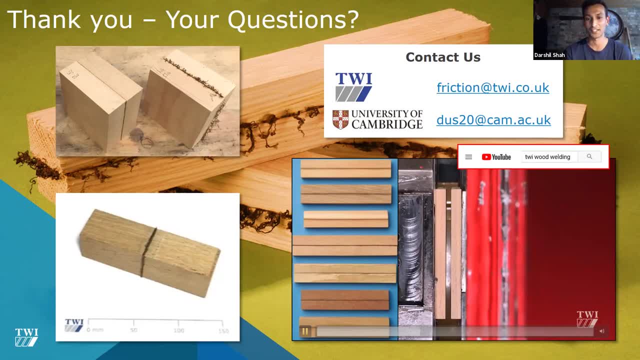 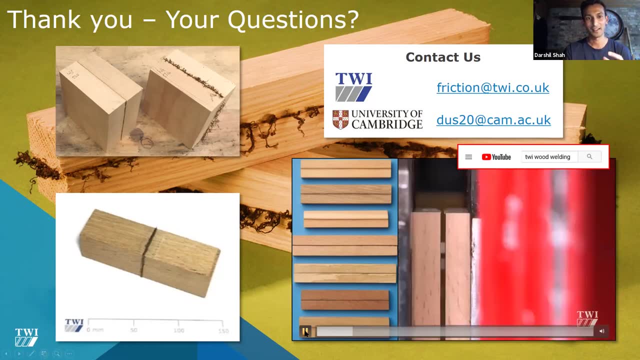 a higher polymer or lignin content, for example, to facilitate that sort of uh bonding. there's also a couple of questions whether you can um join weld woods in different grain directions, and we have um. we have done these on parallel perpendicular to grain, as well as end grain to end grain. 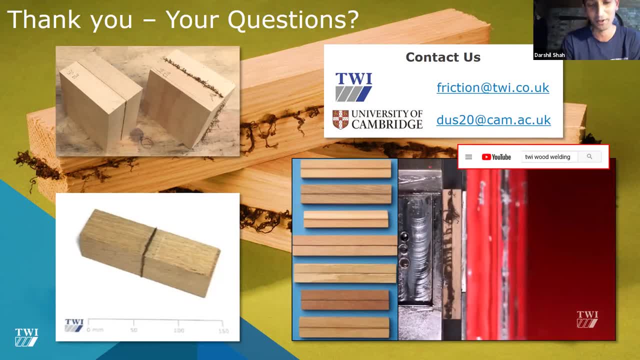 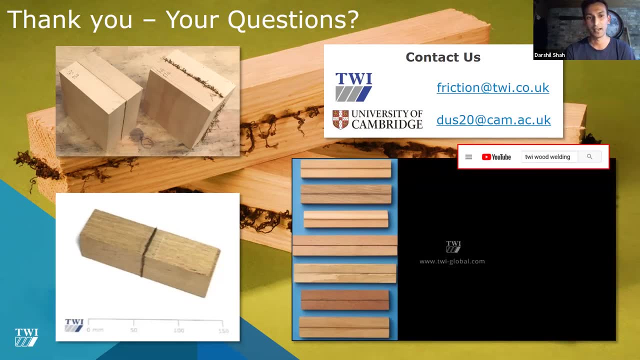 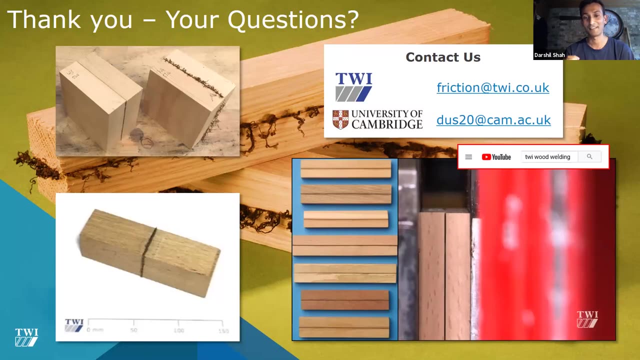 performance is different and therefore, for example, end grain to end grain tends to result in inferior properties in comparison to parallel to grain joints, and therefore it would be interesting also to add how uh we may have to tailor, we may have to select a specific end grain, wood uh to to another. 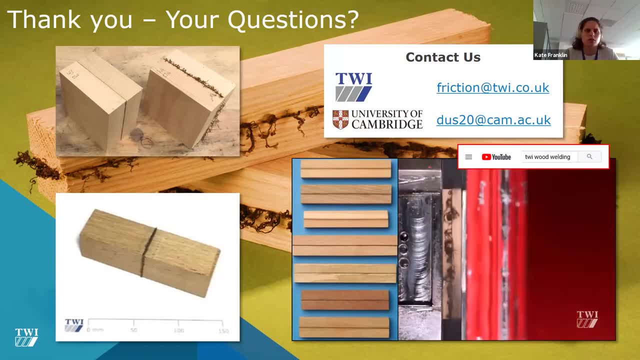 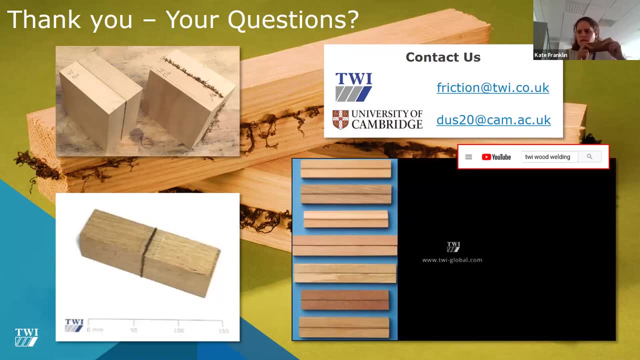 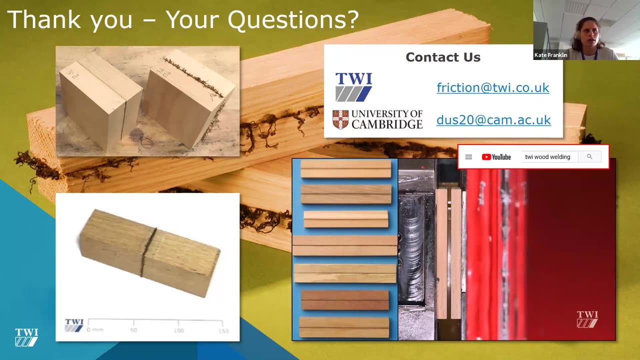 uh, parallel grain wood, for example. yeah, just on on that, note this: the this oak sample, this is what the end to end um, and that's given us really good results. but most of the other work that we've done has has been with the grain rather than entering. 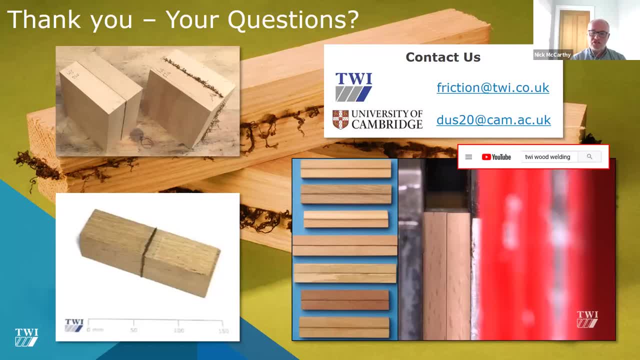 it into the soil. so we're just going to speak a little bit more about what we've been working on, but if you have any concerns or any concerns or questions, you can also reach out to me at the end of the webinar and we'll get to you on the next round of questions.